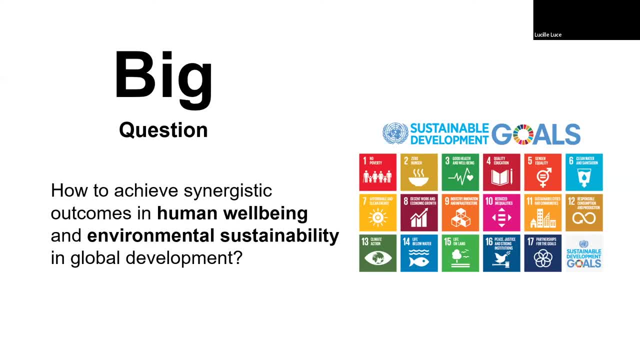 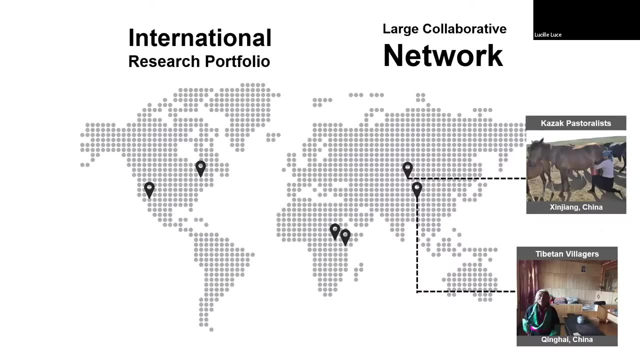 development, And this question is largely aligned with many of the sustainable development goals, which represent a universal call to end poverty, protect the planet and ensure that everyone lives in peace and prosperity. And my work is largely international, which rests on large collaborative 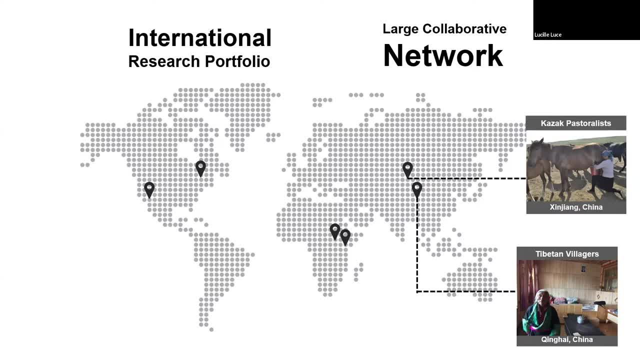 networks, So in Asia. so I worked primarily in Western China, in Xinjiang, the predominantly the ethnic region of China. It's China's Muslim part, like with the Uighurs, Kazakhs. they're studying the pastoral system there And 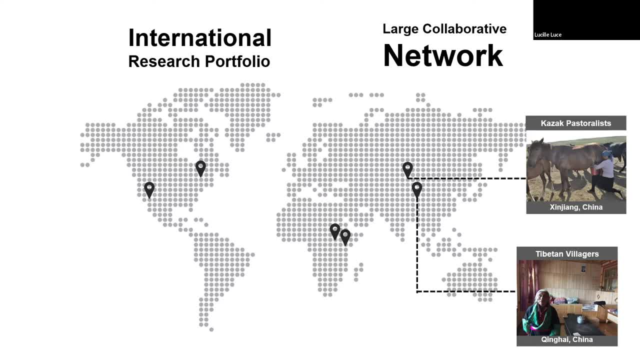 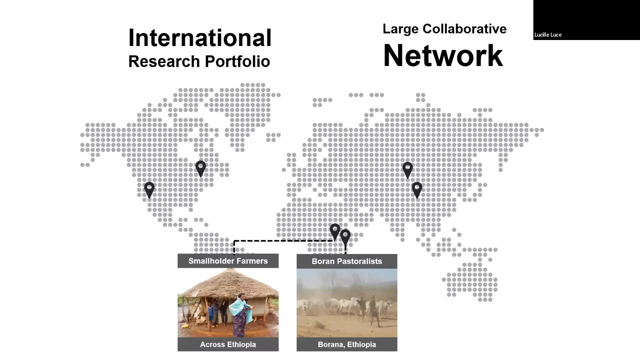 so I'm going to talk a little bit about my research program. I'm going to talk a little bit about my research program And also with Tibetan villagers to study the energy transition process under the targeted poverty alleviation program of the central government. Then in Africa, mostly Ethiopia. So this is my PhD project. I went to southern Ethiopia. 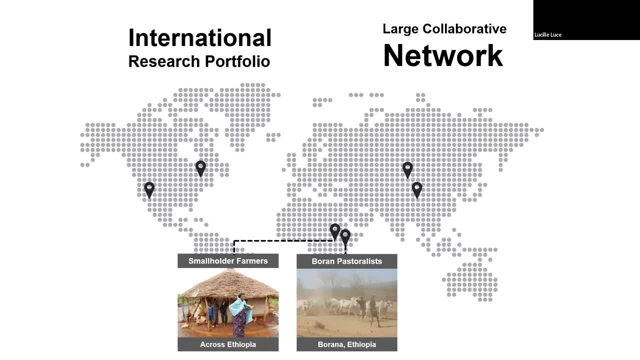 to study the tri-line systems, how pastoralists, their lifestyle, interact with their rangelands, And this started from my postdoc project that started with land tenure change and its consequence on land cover change and smallholder livelihoods at the local level, But later I will also talk about this topic at different scales. 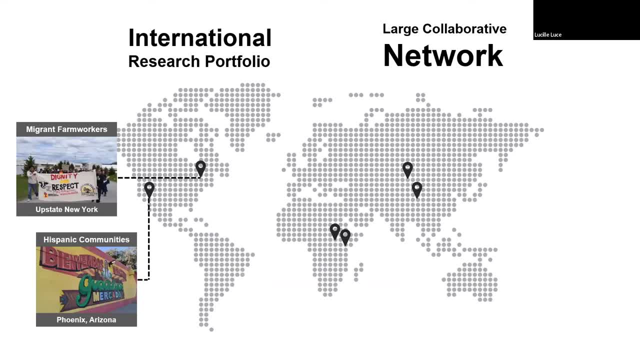 And then in North America, like when I was a graduate student here, I engaged with the farm worker program and went to teach English to these migrant farm workers, for example, Farm workers from Latin America, And among those was the undergraduate students And many of them, like that, I went to teach, like this, the undergraduate students who have 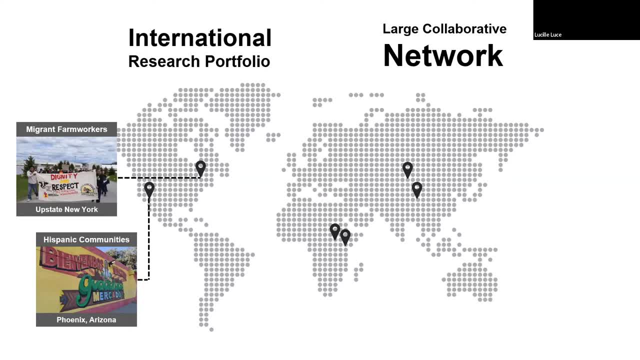 interest in this. they typically speak very good Spanish. So soon after five minutes then the conversation switched into Spanish And because I don't speak Spanish, so I think I fulfilled that goal of teaching English to the farm workers better than those undergraduate students. 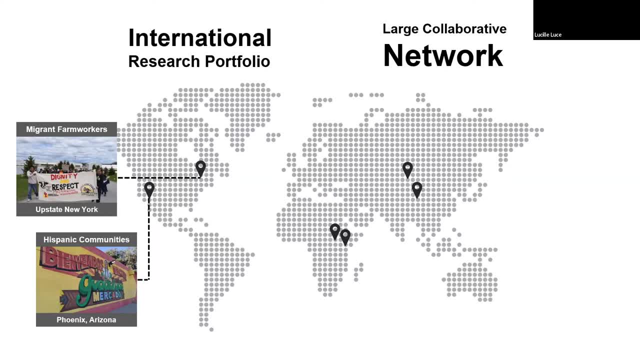 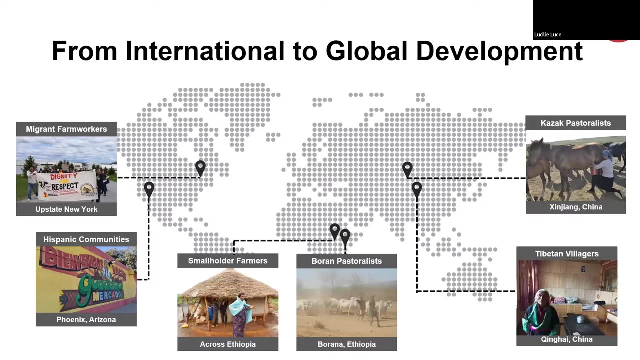 But anyway, so that's my experience with that, And also in Phoenix, like we have some small projects with Hispanic communities, just urban community gardens to enhance local food security and food access, So like as you can see here. so I conducted work in many different parts of 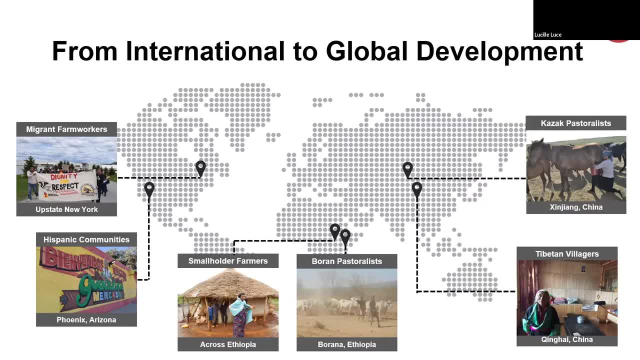 the world. that, therefore, I really echo, is, at least in my field. there is a transition from international development to global development. right Internet we usually think of: oh, development is just out there, It's a question out there, But 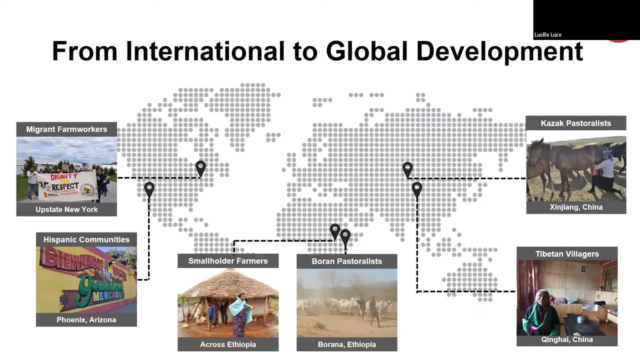 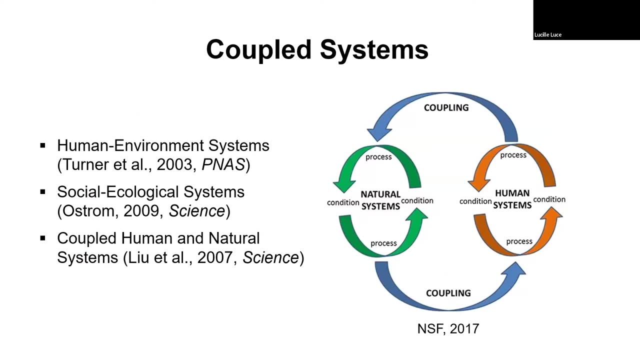 it is a question also, a question right here, right? So that's why I really echo: is this kind of transition And I'm very excited to join a department called global development. So that's some of the background, then theoretical framework. So my research is: 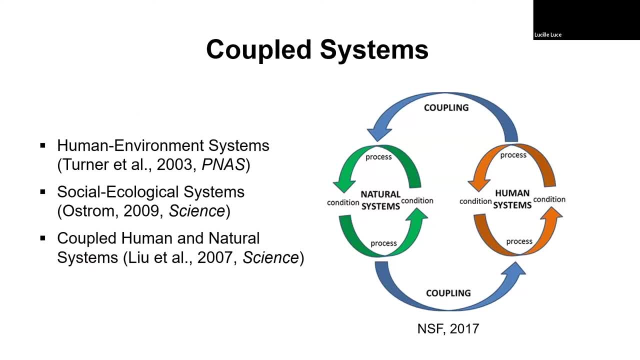 largely involved, formed by this kind of capital system approach, which is also largely promoted by NSF as one of their very few regular interdisciplinary programs. And different terms have been used to name this system right: Human environment, social, ecological capital, human, natural. But at the core of this capital system is about the interactions both within the natural. 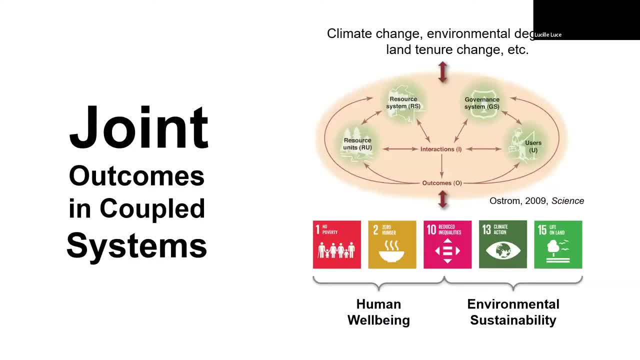 and human system and across those systems. But like moving that forward, like I think the recent frontiers of our study in social ecological systems, is to analyze the joint outcomes right. So when there's interactions like, what's the implications on human well-being and 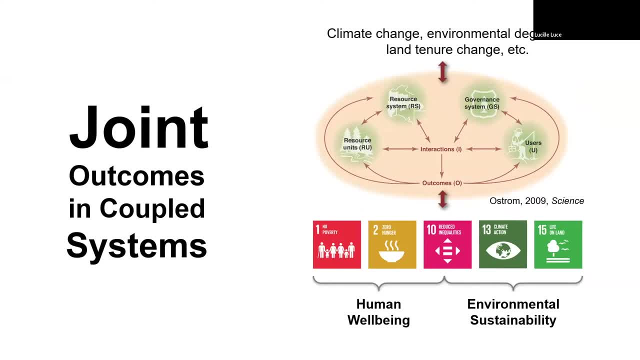 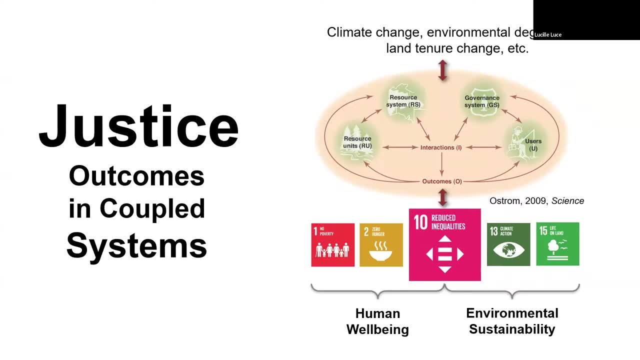 environmental sustainability in the context of climate change, environmental degradation or land tenure change. But I would also highlight that actually the justice outcome of all those kind of interactions is gaining more and more like attention and and significance in recent scholarship. So I will also talk about later in my talk how 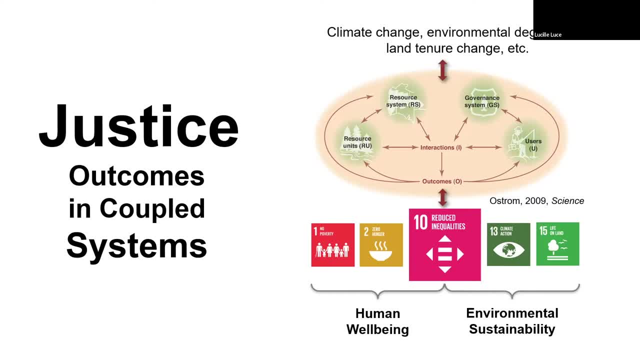 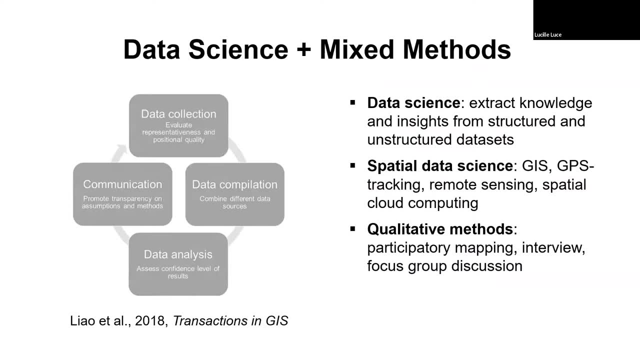 this SDG 10 is considered in my work And then just one slide on the methods. So I use data science and also a different, like mixed methods to answer the question of environmental sustainability, on how to achieve synergistic outcomes in human well-being and environmental sustainability, and especially many spatial data science. 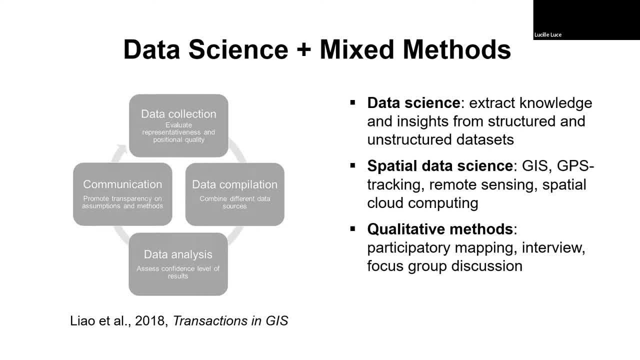 methods such as GPS tracking, GIS, remote sensing and some spatial cloud computing methods, And I also do qualitative work. I go to the communities and do participatory mapping, interviews and focus group discussions with smallholder farmers and herders to triangulate, like the knowledge we extract we get from this more quantitative method. 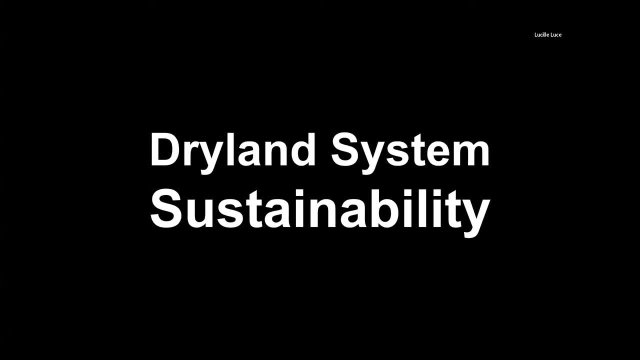 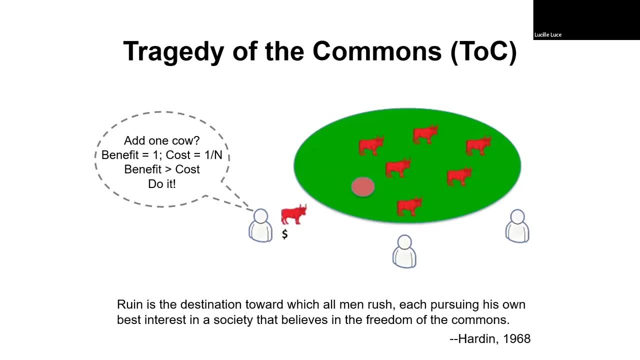 So first topic, dryland system sustainability. Okay, So my interest in this topic started from my learning of the tragedy of the commons when I was starting here. So according to James Harden, so ruin is the destination towards all man rush, each pursuing his, at that point only his. So this is a direct quote. 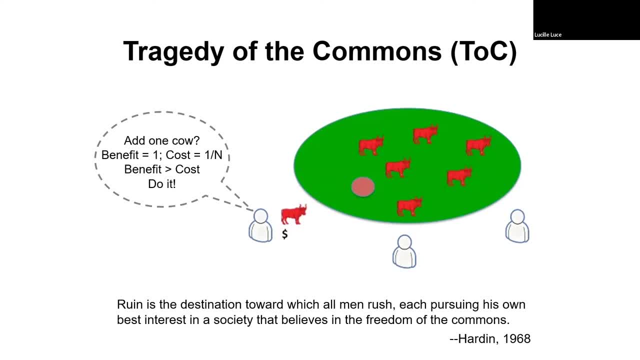 his own best interest in society and believe in the freedom of the commons, So utilize this to So. the pastoral system is a very classic example of tragedy of the commons right, Because every herder using that same patch of pasture, anyone will have an interest to add more cows. 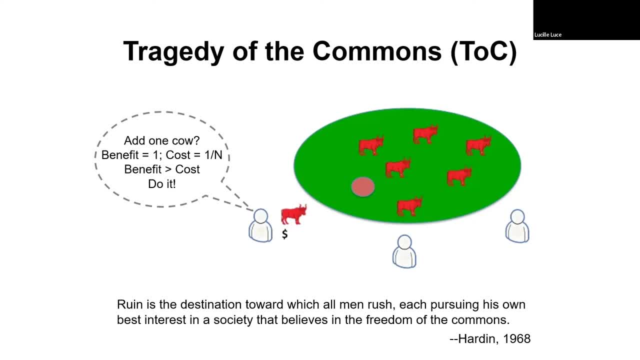 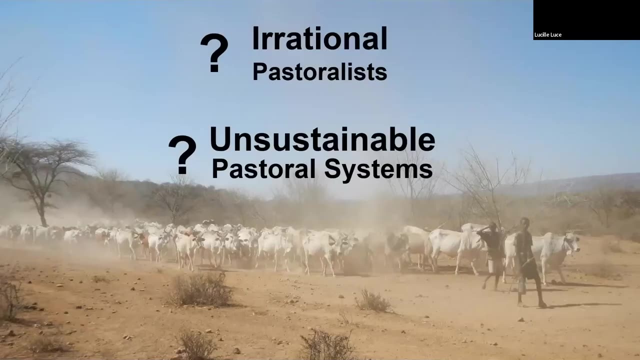 to the system because the benefit is always greater than the cost. right Benefit is one, cost is one over n right Shared by everyone. So why don't I keep doing that right? So that's Hardin's argument. And looking at a photo like this: 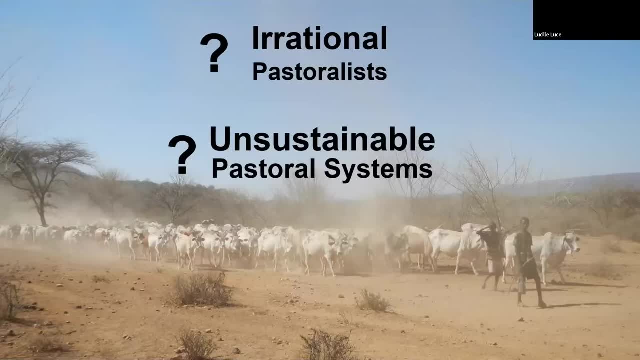 so people are more likely to be convinced by Hardin's argument. right, Because pastoralists, they are irrational and then that will eventually lead to unsustainable pastoral system. So this is a picture I took in my field work in Southern Ethiopia And I would say this is a little bias. 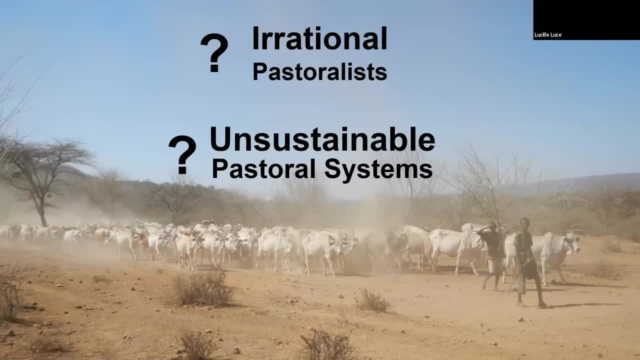 to capture what's going on in the system, because, as scholars, we always go in the dry season, Because if you go in the wet season your vehicle will get stuck And you don't want to call another vehicle to save you, and then you go back in the months. 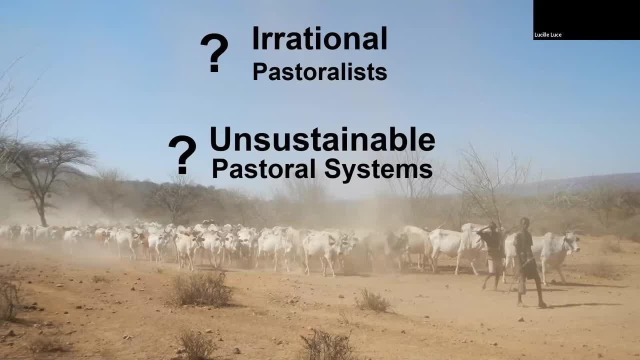 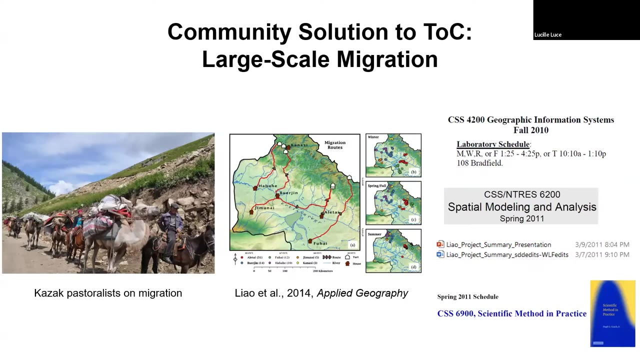 and then say that's a stock vehicle, right, So it's very biased. So I only returned in the rain season once and the landscape looks totally different. Okay, I just want to highlight that And the solution to the tragedy of the commons. 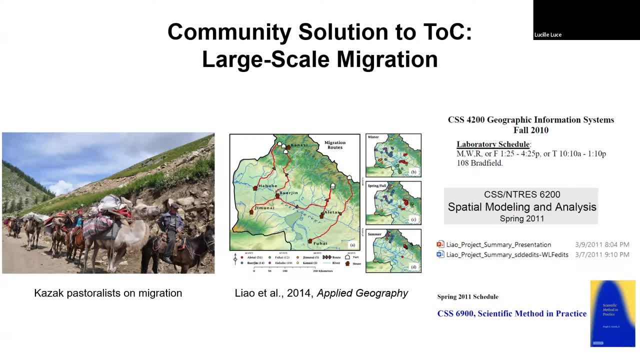 is a large scale migration. So this is in far north-western China. The cattle pastoralists migrate between the Gobi Desert and the Altai Mountains. that cover a distance over, in some cases over 300 kilometers, one way from the desert to the mountains. 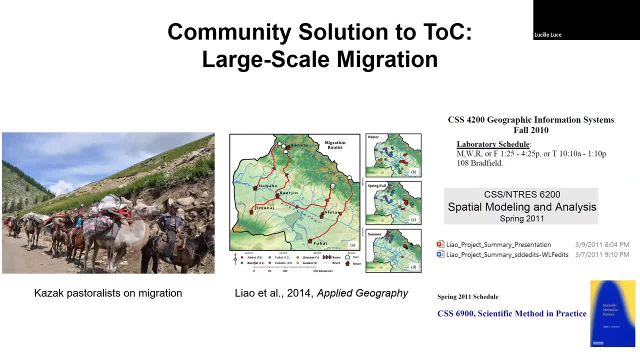 And so this is a place like throughout my talk I will mention, like how my interaction with SIPs- or at that time we called it CSS. right, I took many CSS courses, especially with Professor DeGloria. He helped me a lot. 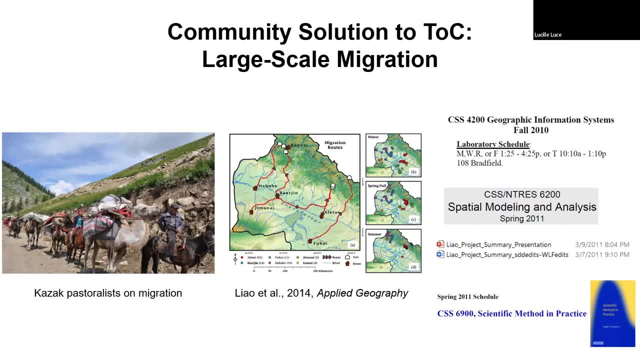 In those kind of work. And I still remember in my first semester here I took his GIS class And then the following semester again took his class spatial modeling and analysis. Probably this is a map like I created, like in his GIS lab. 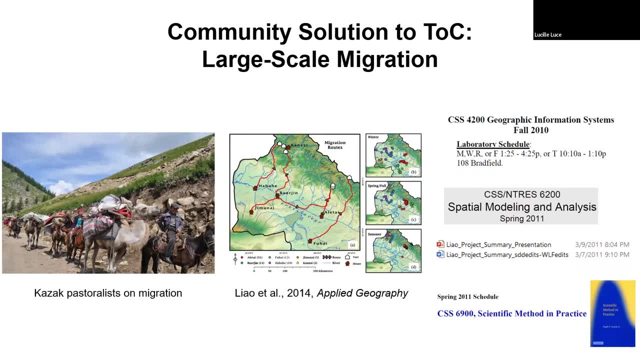 Sometimes I sneak in to the Bradfield lab because natural resources graduate student- at least me, some of them, like including me- were assigned to the chicken house, F house, whatever we call it. It's very hot and humid when the temperature is around 30,. 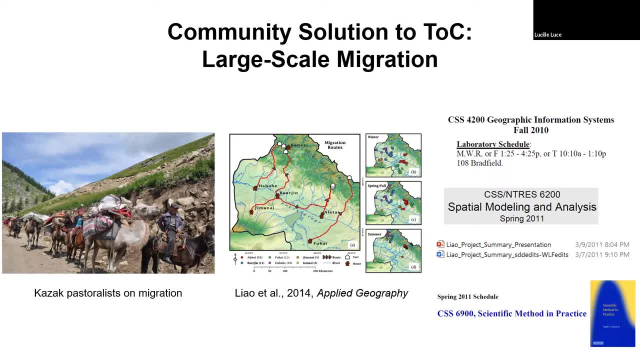 oh, like centigrade. So that's why, like, I like to use the facilities there And then you see, like this SSD edits right. He put the like he gave me some like feedback back in like 2011.. 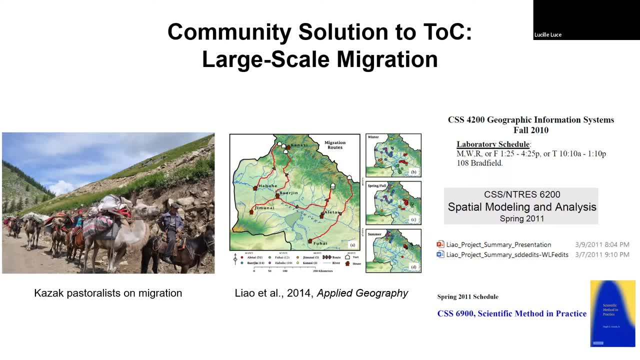 So this morning, as I was preparing for this, I'm like: Oh, Steve helped me, like when I was preparing the field work. Yeah, exactly, And this morning, as I was preparing for this, Like oh, Steve helped me When I was preparing the field work. 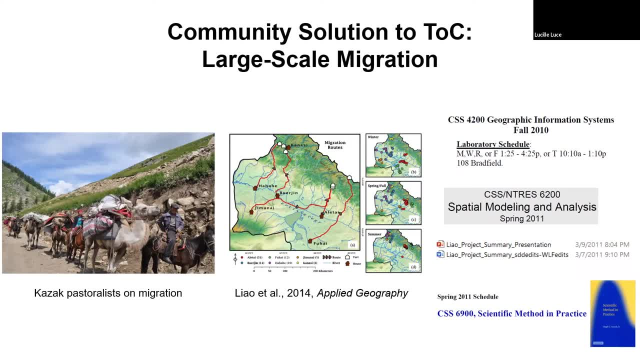 coming up with my ideas. right, those are two courses I took with Steve and another one is CSS 6900, the scientific methods in practice, and which is a co-taught by Gary. he is already emeritus now, but he said in my class I'm basically a TA for for the author of this book, which is Hugh. 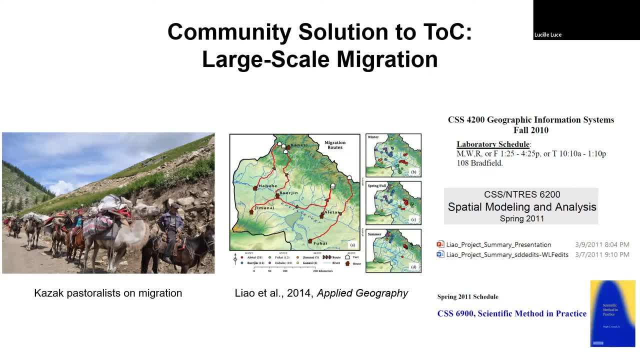 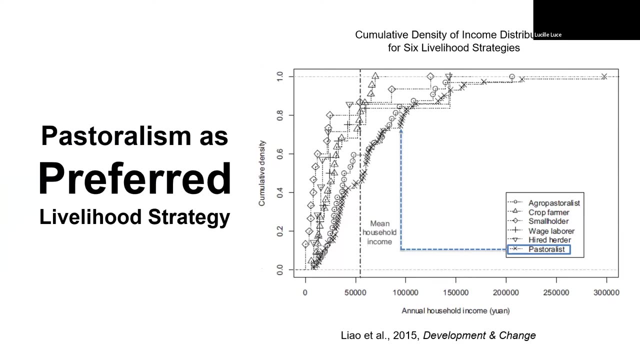 Gao. he wrote this book and throughout the semester it was him was teaching this class. so it's, it's a, it's really a, like a philosophical reflection of scientific methods which inspired me a lot back then. so just a little story there and then, okay, back to the topic. so large-scale migration. 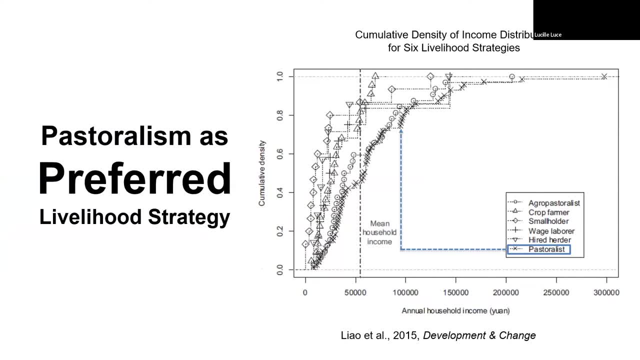 as a solution, right, right, but pastoralism actually, as is the, is the is the, at least in the context of a far north western China, pastoralist pastoralism is a preferred livelihood strategy because if you just we look at the annual household income, right, it just dominates all other, it is just preferred. 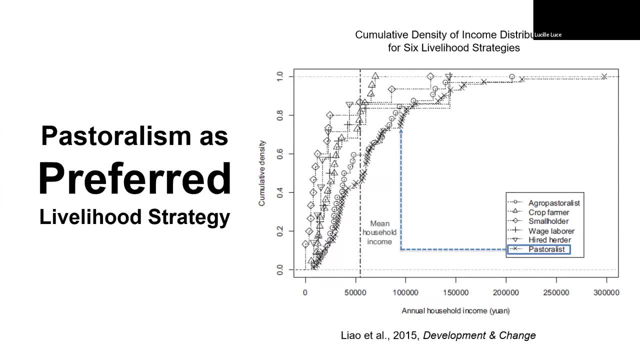 come. it's higher compared to all other five livelihood, like strategies such as agro, pastoralist, crop, farmer, smallholder wage labor and the hired herder. but even given, even if so, like the government's, like their own government, they are the ones who are the ones who are the ones who are. 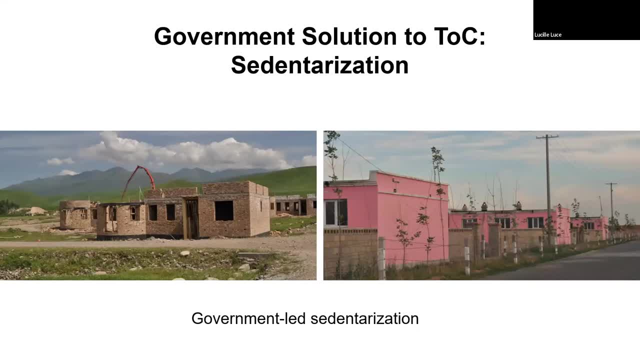 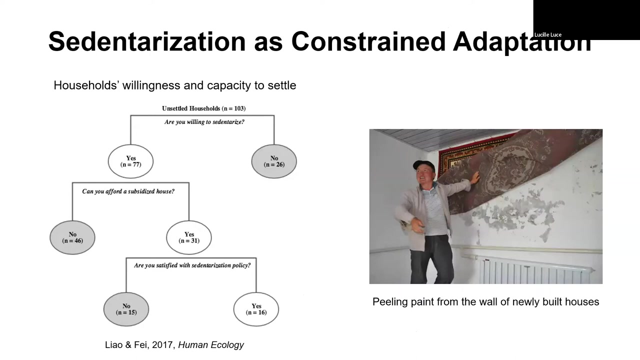 their solution, right in in the Chinese context, is to sedentarize them. they construct this sedentarization villages and subsidize them. let's sell them to these herders at a lower cost as an incentive to convince them to move into those villages. and one in our, in our, like a survey with those herders. we do see that, actually most, you see. yes, on the unsettled households like our here in mid south east us. in ahuast in manila. it questioned children. lives are very little and children one, one hundred five people and one 94% of the children is enslaved and they're just hair daling on their hair. numbers of four are at almost EVERY student. 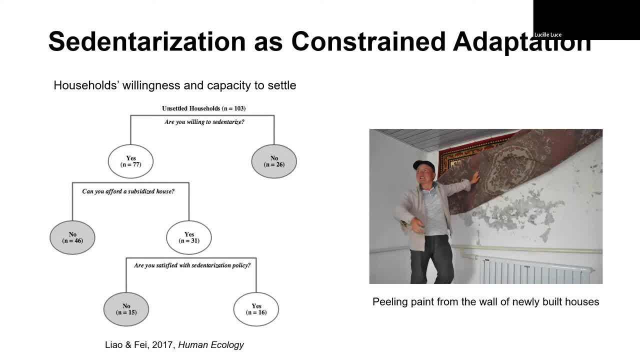 28 percent monthly. same set, six point helms, a hundred percent of the labor and farms in skin and feel the same thing like for the unsettled households, the majority of them. they do want to settle, They want to move into the villages because they know. 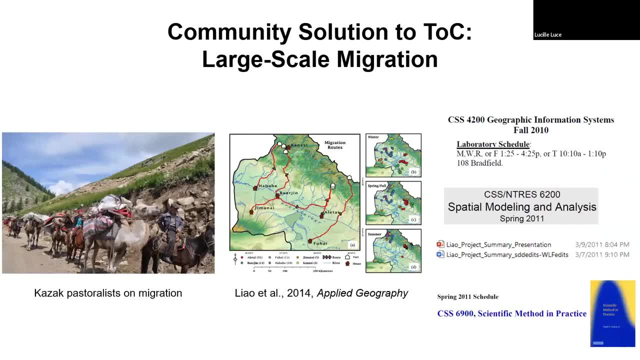 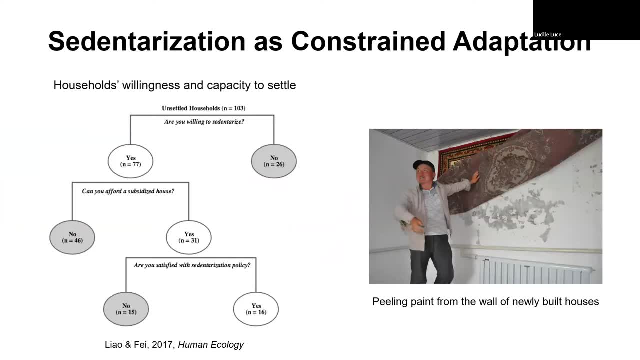 doing this kind of large-scale migration is not easy, especially in the context of climate change, environmental degradation. But their experience after they moved into the houses- you see this peeling paint from the wall, The poor quality of those houses- are of critical concern. 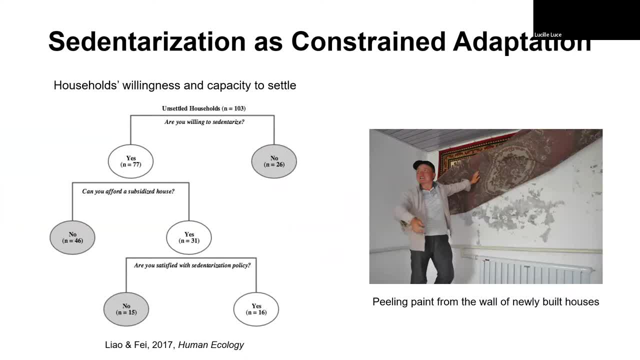 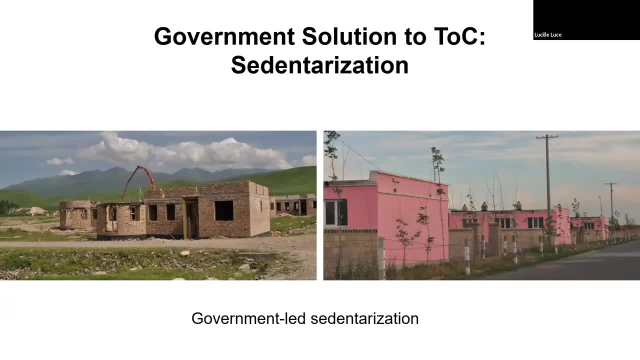 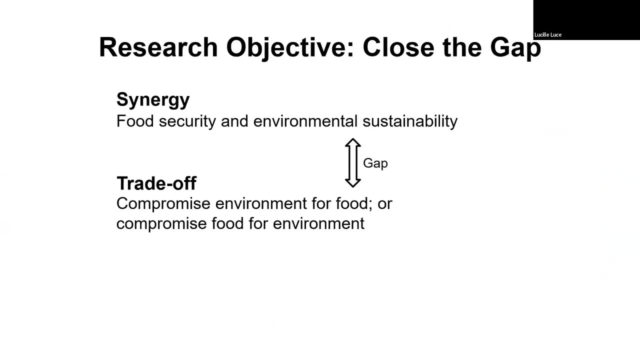 And this is just one example. And finding viable livelihoods are like in those sedentary villages is also very hard for them because, many of them they do not have the skills to transition into non-pastoral livelihood strategies. So therefore, the gap between the synergy states. 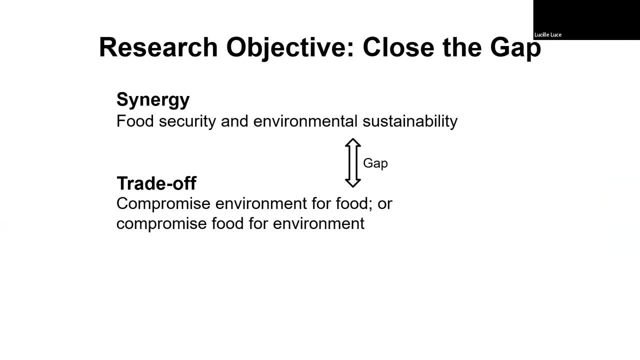 like food security and the environmental sustainability with the reality, which is a trade-off- either compromise environment for food or compromise food for environment, motivates me to like. I think it's important to address, But what's more, what's worse on the ground. 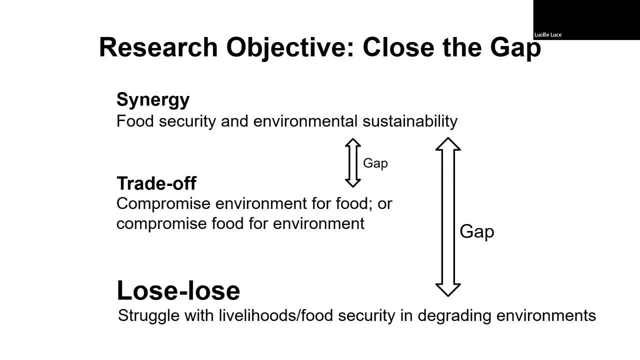 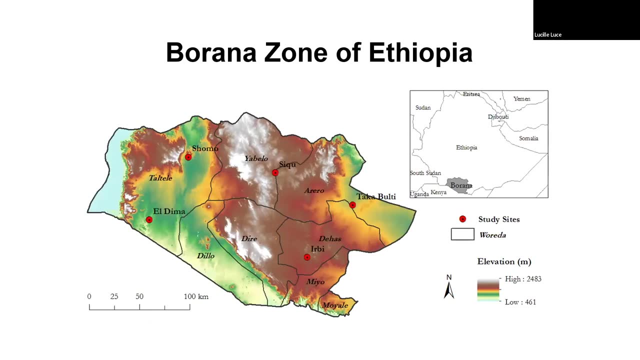 is a lose-lose scenario where we see, like for example in Xinjiang, people, the herders, they struggle with their livelihoods, integrating environments. So closing these gaps becomes a fundamental goal in my research. So then, after I did my masterwork in Xinjiang, 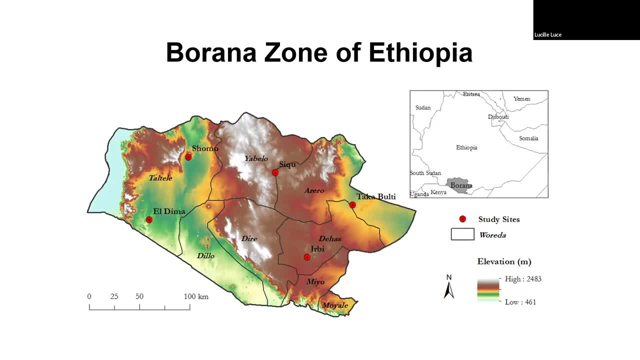 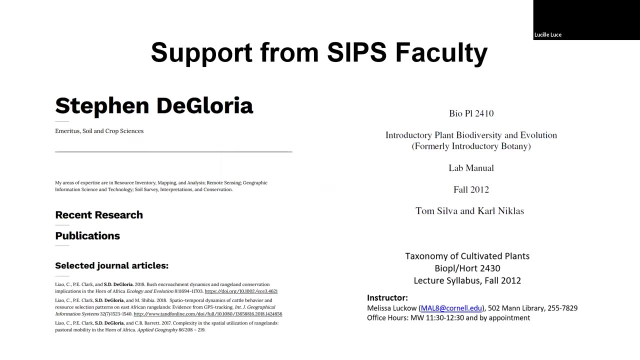 then I went to southern Ethiopia to do more. So this is five of our study sites in the Burana zone of Ethiopia, which is just north of Kenya. So again for my PhD project I received even more support from SIP's faculty, especially from Steve. 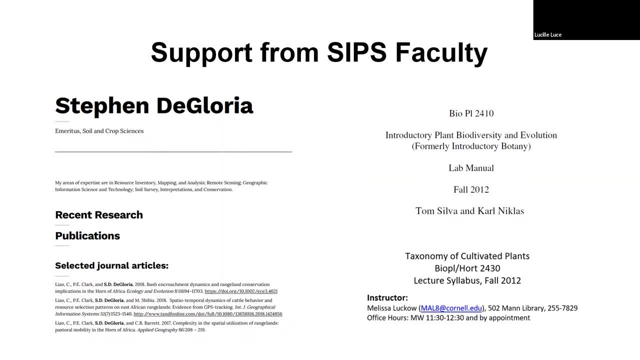 The first I remember when I started my PhD. I asked him, Steve, can you serve on my graduate committee, PhD committee? And he was like I'm going to retire, But now when I finished, he still hasn't retired. 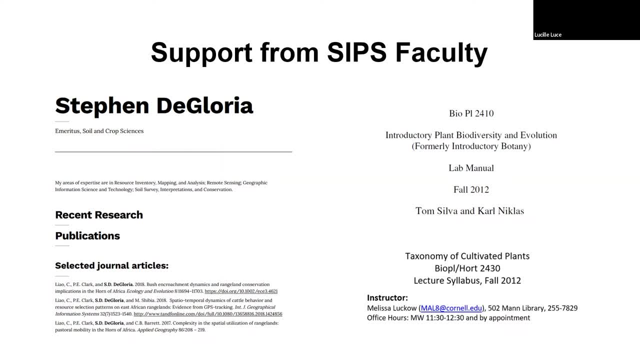 He said he was in a phased retirement, but I don't remember exactly when he retired but he was still here, But anyway, so you see some of his most recent publications Before he retired was with me, so I'm happy to see that. 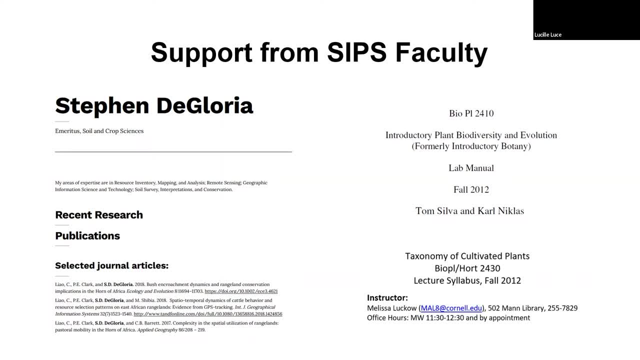 And later he actually applied for funding to support the GPS tracking of the cows in southern Ethiopia. So that's supported by Steve and also I took two classes, Thank you, Thank you. So my first class was in SIP, so one by Tom Sylvia. 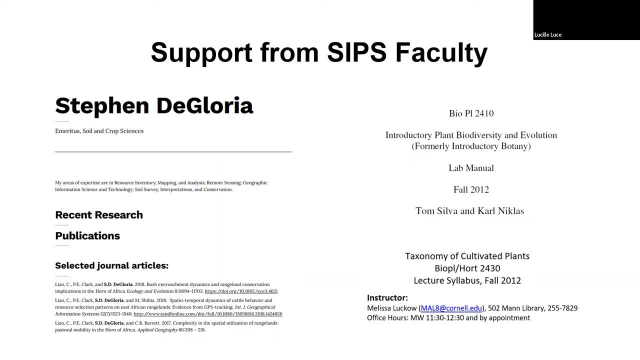 and Carl Nicklaus. That class was in this classroom. I still remember Professor Nicklaus. He was doing this. So he draw like a flower structure, like with two hands, something like that, making it very hard for me to keep up with his pace because he used two hands. 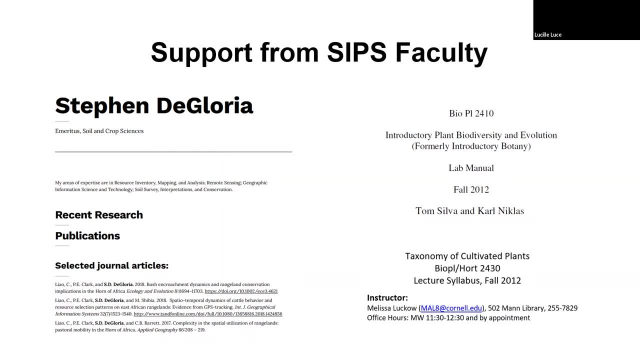 to draw those structures. But it's really amazing to see how he do this kind of things. And another class I took was with Melissa Luko on the taxonomy. I took those class because I wanted to identify the scientific name of plants in Ethiopia in my study area. 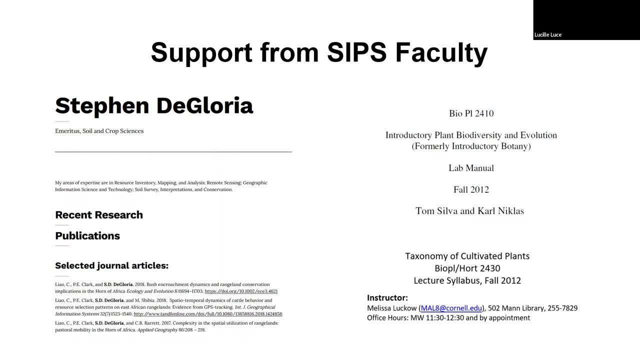 So it's quite like a challenge for me to take those and then do the field work and bring the plant specimens to the national bearing of Ethiopia and Judah and identify the scientific name. That took quite a long time, especially for someone who didn't have much training. 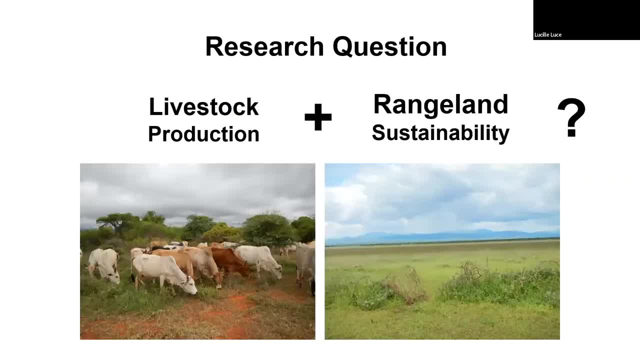 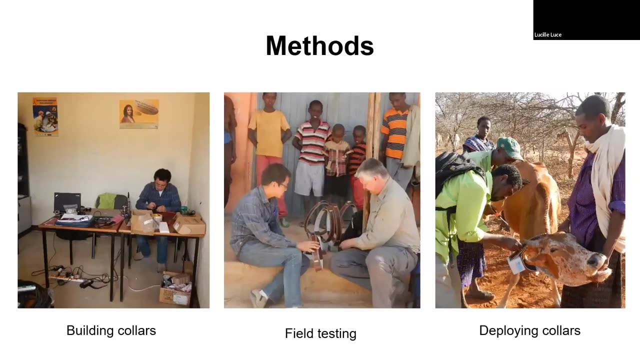 before then on this topic. So the research question about achieving synergies, which is in that context. synergy means the lifestyle production and the rangeland sustainability. We need to have both Methods. this is well. I would say this is one of the novel. 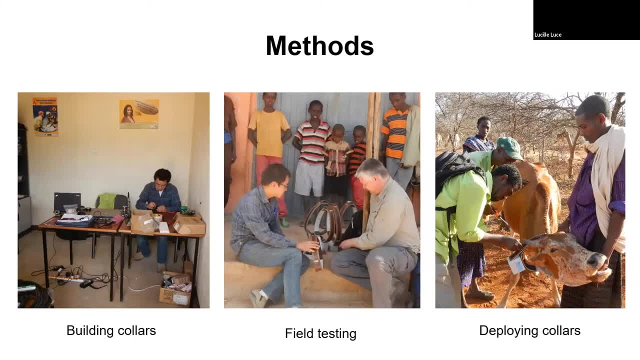 approach we did in that project is the GPS tracking. So Steve was a major PI in this effort. So this is our collaborator, based in Boise, Idaho, is a range scientist. He designed those GPS collars and shipped them to Ethiopia and we put them together and deploy them on the cows. 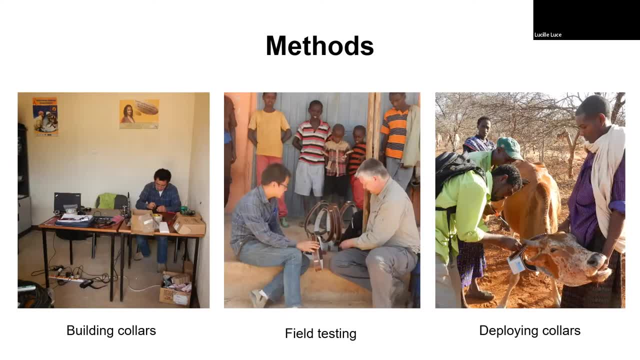 In total we did. we put our GPS collars on 60 cows in five study sites for four years Every five minutes. we got like a coordinate, like update. So that means over millions of points right. That has spatial and temporal information. 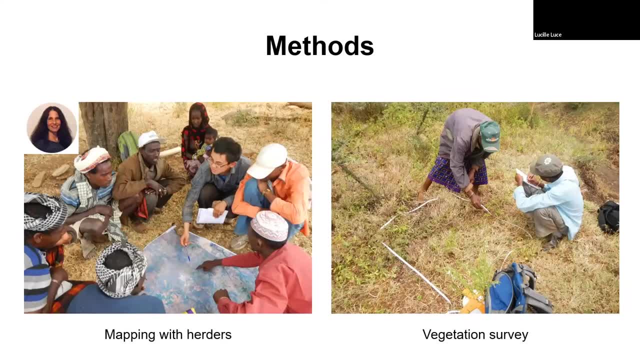 And in addition to that we did mapping with herders, and Magdalene she helped me with preparing those maps. So lots of support from CSS herders Back then. and then we also did a plant survey to study the rangeland vegetation. 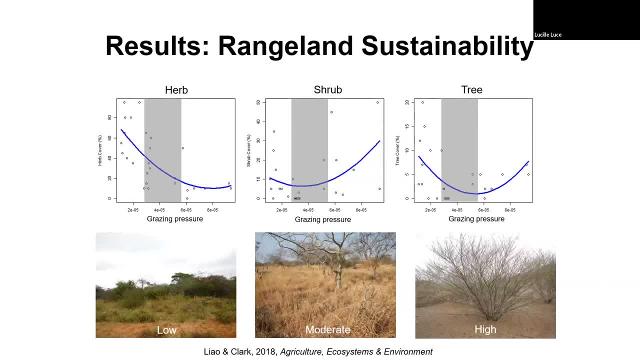 So now some results. So for this one. so we see on the rangeland side. so I'm just using one slide to summarize What we see is like moderate grazing pressure contributes to rangeland sustainability in the sense that it has the dense herbaceous cover. 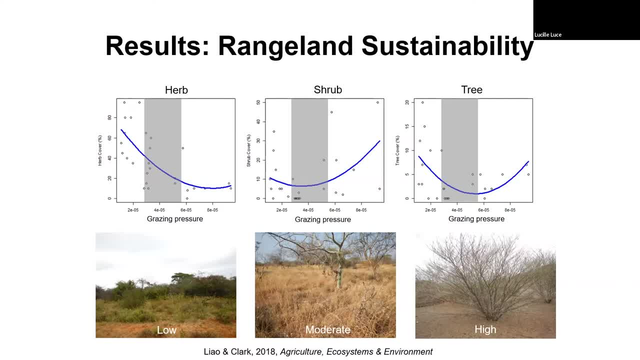 out of sparse woody plant cover, But when the grazing pressure is too low the system tend to shift into this kind of dense, dense herbaceous cover. It's kind of dense thickets right, And the cattle will have a hard time. 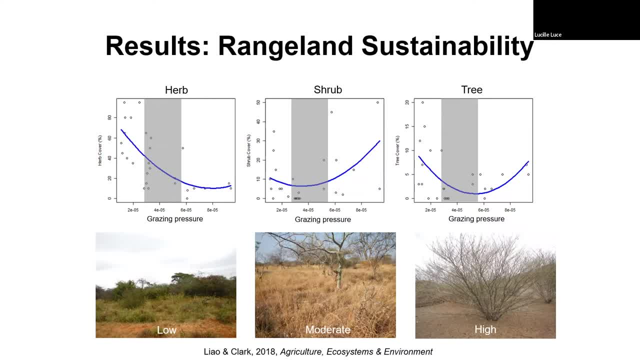 to access the herbaceous resources in the understory. But when the pressure is too high, right, The system tends to shift into this bushland, right. Very little herbaceous stuff for cattle grazing, only those kinds of acacia shrubs. 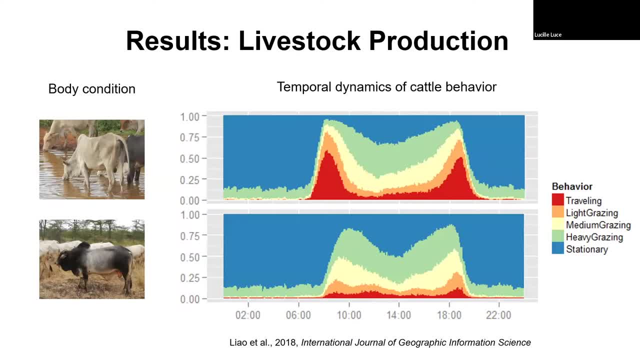 And on the other hand, the other synergistic goal is livestock production. So when we think of a livestock production outcomes, you think about the body conditions of those cows. right, Not good, good Like thin ones and fat ones. Those are from the herders perspective. 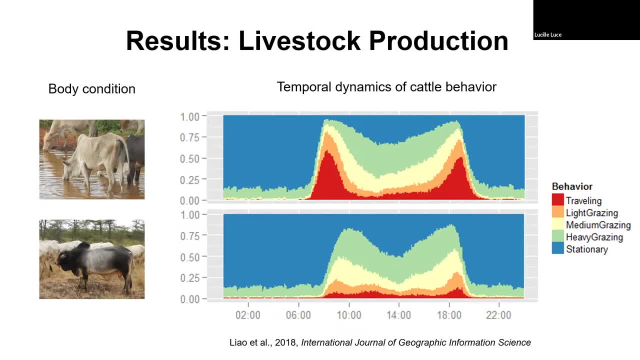 they will think like that. But of course we didn't measure their body weight change over time, right. But with GPS tracking that can shed light on the livestock production outcomes, right. So I'm just here putting two cows: temporal dynamics of their behavior. 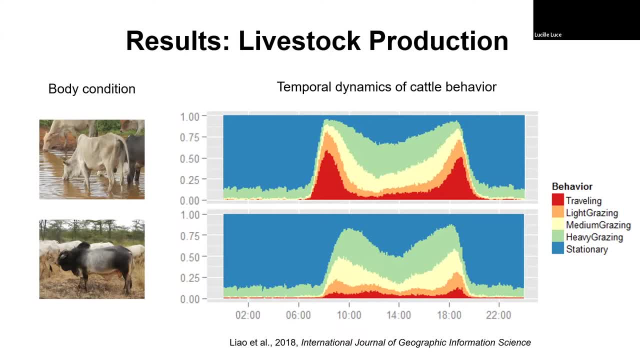 So the top one you see spend a lot of time, effort, effort. So the top one you see spend a lot of time effort. So the top one you see spend a lot of time effort Traveling. that means fast moving from in the morning. 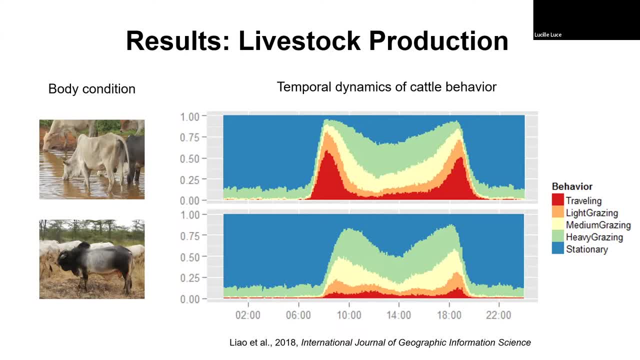 Traveling that means fast moving from in the morning and afternoon, late afternoon, to rush between the camp location, Their base camp, to this major grazing sites. go there fast and then come back, But during the day they will have opportunities to graze. But during the day they will have opportunities to graze. 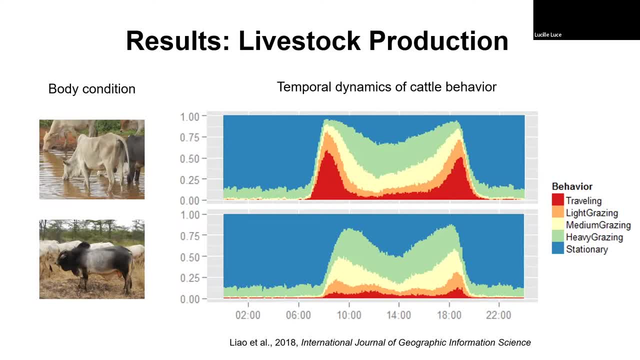 But this one below belongs to the owner- is a mobile herder, right. That means he relocates his cow to different locations in the dry season. So yeah, during the day of our camp relocation you do walk a long distance, But once you relocate to a seasonal grazing resource, 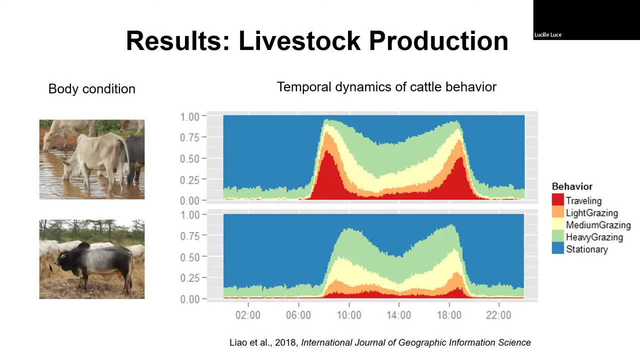 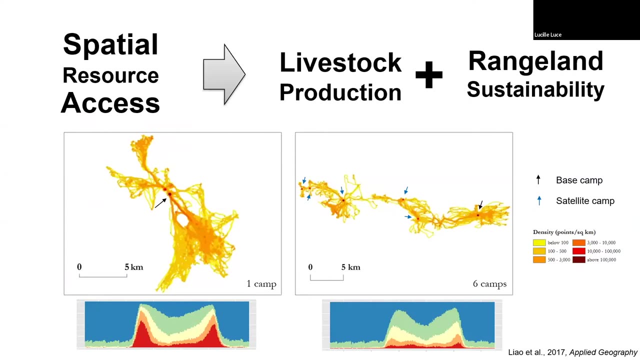 then you, basically the cattle, wake up and they start to graze, So they can minimize the traveling behavior throughout the season. And if we link those temporal dynamics of cattle behavior to their spatial utilization pattern, we will see that the one owned by a sedentarized herder 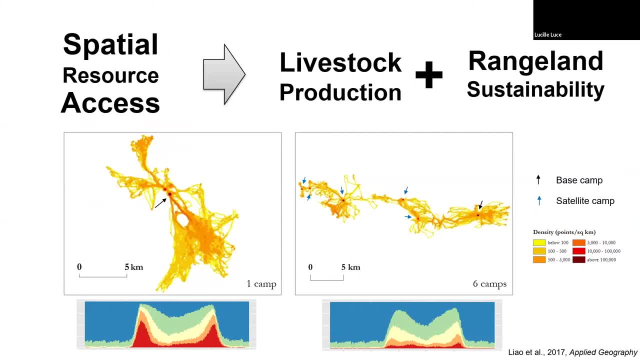 this is a base camp location And as it gets drier the cow needs to walk longer distance Or towards the other side. this is in the mountains. That means the cattle need to even climb up the hill to access the resources. But on the right side camp relocation. 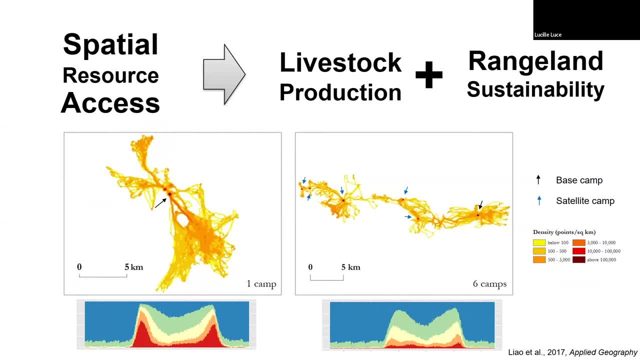 really help with minimizing traveling behavior. This is a base camp location. In the west season, the cow is based somewhere here, And then the dry season comes, the cow is relocated to different patches for a range of resources. So that's why we see this. 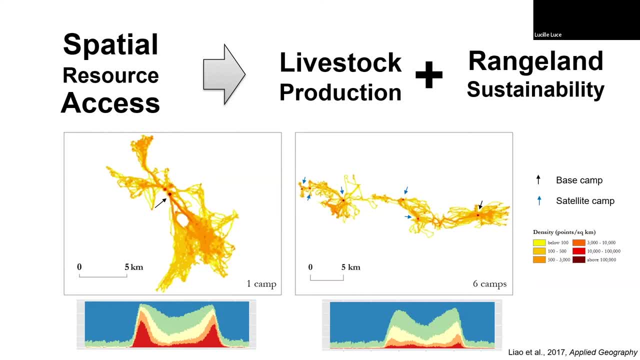 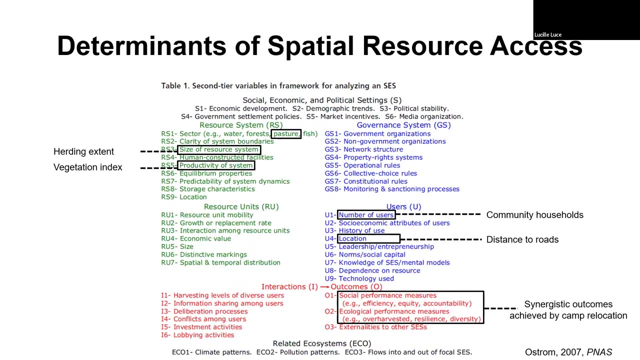 So the take home message here is that spatial resource access is key, is crucial to achieve synergistic outcomes in that, at least in that context. So the next question is: what are the determinants of our spatial resource access? So here I'm going back to Ostrom's theory. 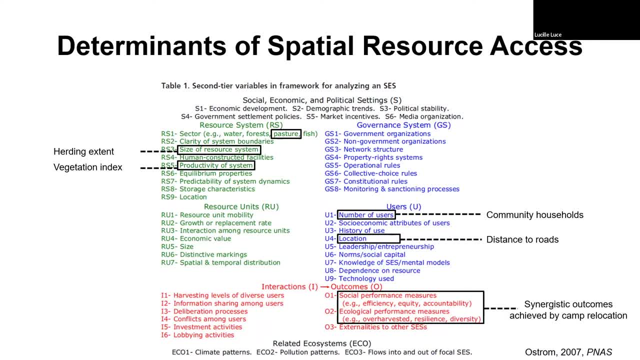 like second tier variables in the framework for analyzing a social ecological system. So obviously I didn't have data for all the variables that she identified, but, as she said in the paper, it's okay, so you just get as many variables as possible. 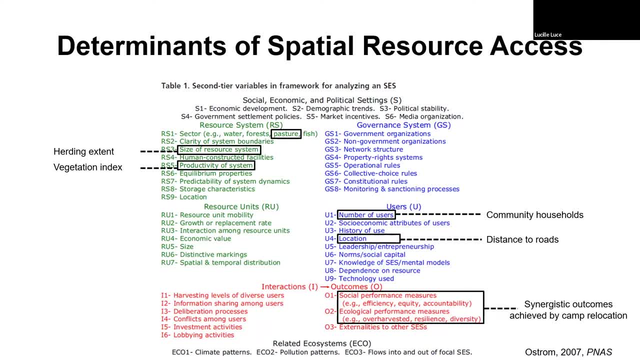 So for me it's a pasture system and the size of a resource system. I use the herding extent to measure this and the productivity using vegetation index. And for users, we have a community number of households in a community and location. 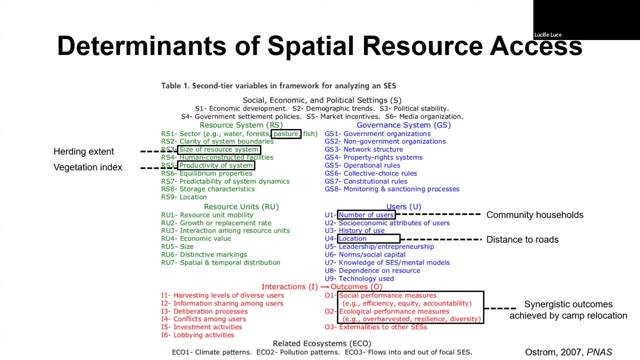 we use distance to roads as a measurement And the outcome here is a synergistic outcome achieved by camp location. So here I'm skipping like the big regression tables, and just to show you the significant results. All those predictors have a significant effect on this outcome. 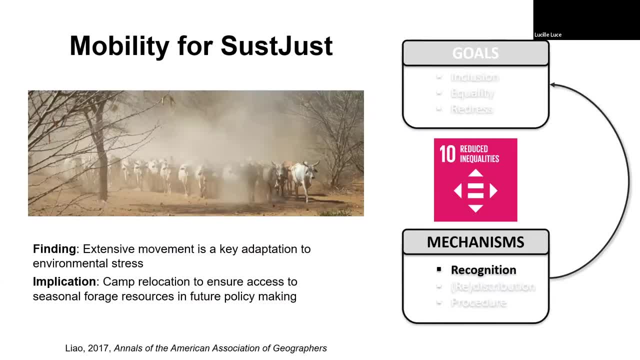 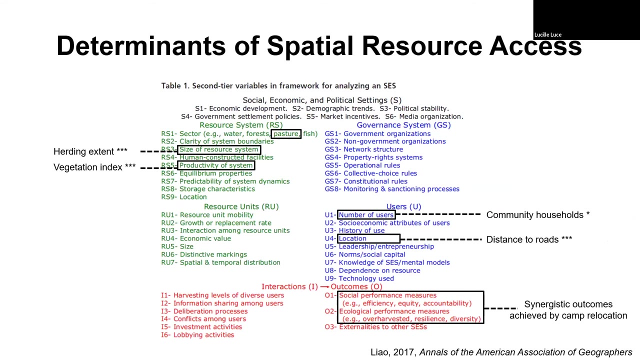 So, but I will just say explain more in here. So the implications. So, first of all, we find, as the extensive movement is a key adaptation to environmental stress, That means this is the one from this vegetation index. As the vegetation index goes lower, 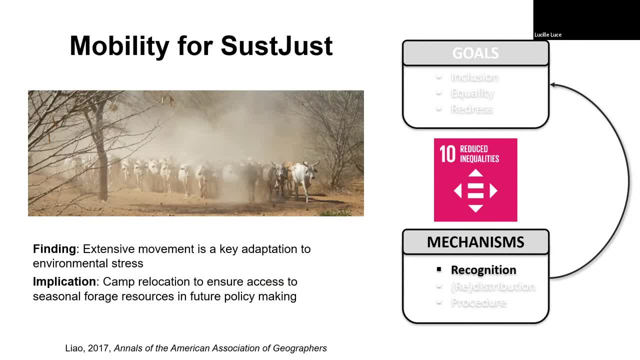 pasture is more likely to decrease, It's more likely to do camp relocation right. This means it's a clear adaptation to environmental stress, and policy implication is that camp relocation should be recognized as a key strategy to ensure seasonal access to forage resources in future pastoral policy making. 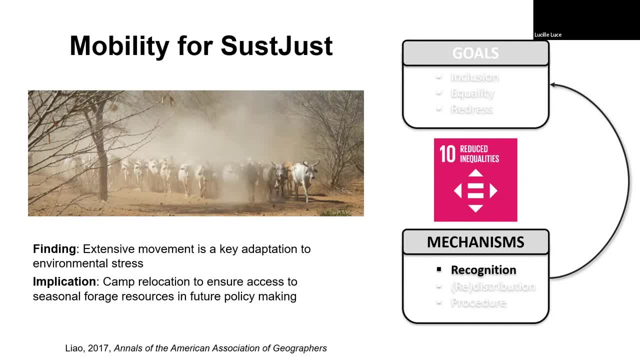 instead of encouraging this kind of sedentarization policy. So here I didn't mention is like same as in China. the Ethiopian government is also, you know, is also encouraging sedentarization. They didn't have the like the resources of the Chinese government to subsidize the construction. 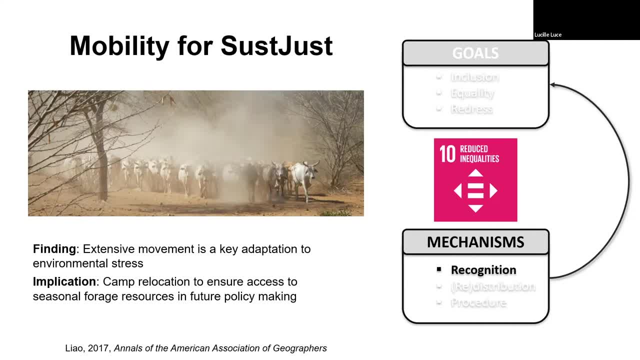 of sedentarization villages, but they give land to people as an incentive, say, hey, if you're sedentarized in this village, you can enclose this much of land and that's your private land for crop cultivation, right? They are trying to give incentives. 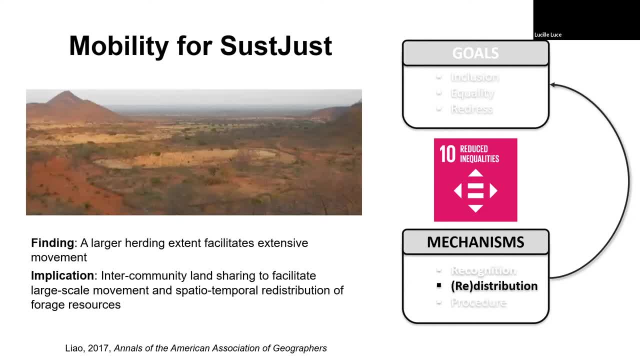 to encourage certain behaviors. And second is related to you know. it's also about, you know, related to the resource herding extent here. So of course, right, a larger herding extent can facilitate extensive movement. but in this part of the world, the pastoralist, 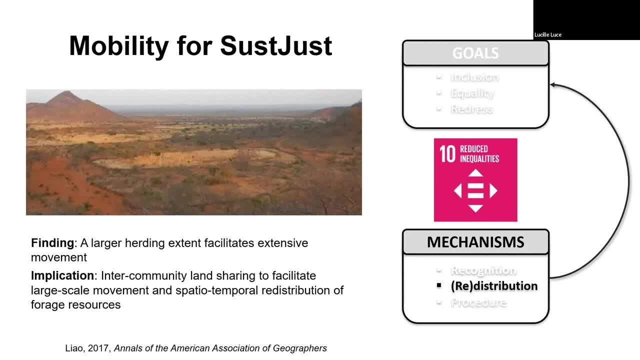 given the increasing population- livestock and human population it's the herding extent is shrinking. So one potential solution to this is to facilitate inter-community land sharing to facilitate large scale movements and spatial temporal redistribution of resources right on a reciprocal basis. 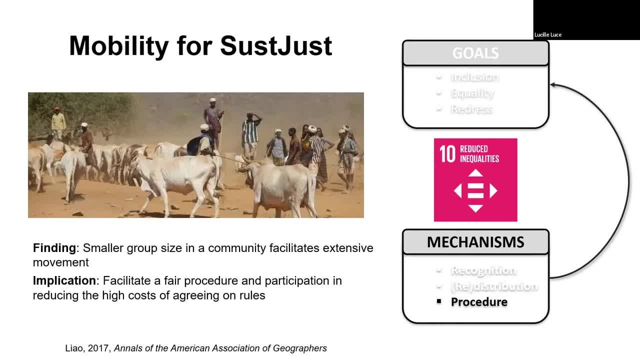 And the third is that it's about a group size effect. A smaller group size in a community facilitates extensive movement. So this means that the effect of group size on the transaction cost of extensive movement is negative And this means that in the future policymaking 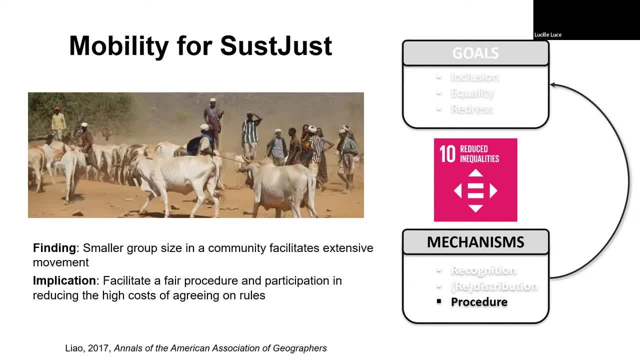 we need to facilitate a fair procedure and participation in reducing the high cost of agreeing on rules to coordinate this resource sharing. camper, location And this: as you can see, there is a conjunction in the access to water. This is a borehole, like pumped water to water the cow. 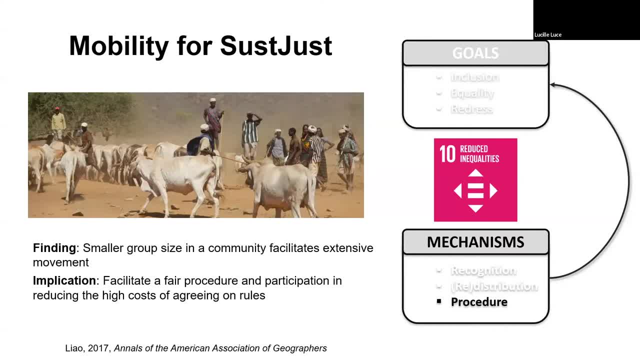 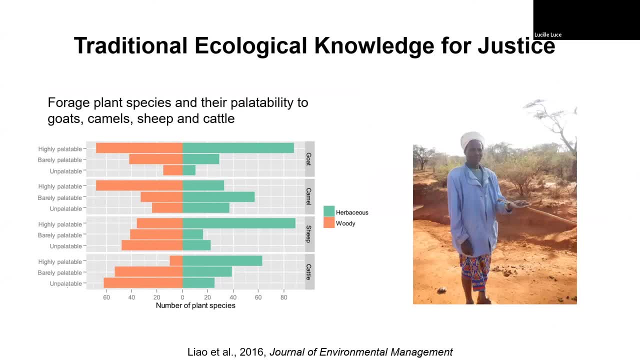 Especially in the dry season, it's necessary to water the cow at least every three days, Otherwise they will be in trouble. So in addition to this kind of a GPS tracking, a related research right, we also studied, I also studied. 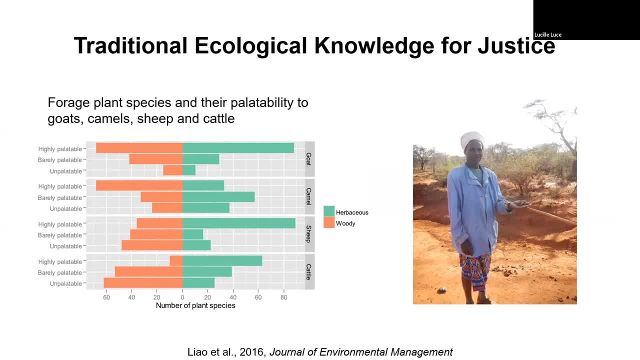 our traditional ecological knowledge like basically to study the palatability of different forage species to four major livestock species in that part of the world: Goat, camel, sheep and cattle right. So either herbaceous or woody, or the palatability level. 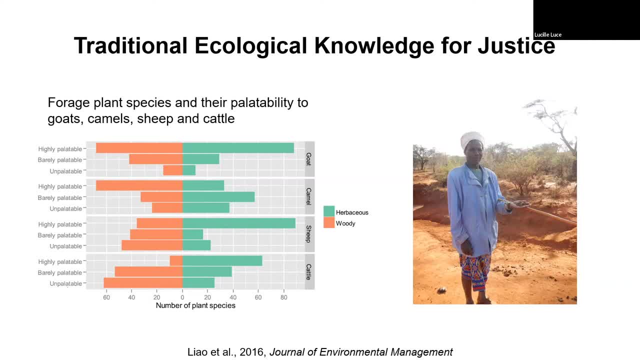 So this is the hard part, right, While I'm preparing, I did took those plant science class because I wanna do this. So collect like the plants, like specimens, right, And bring them to the National Barium of Ethiopia. Meanwhile, when we collect each specimen, 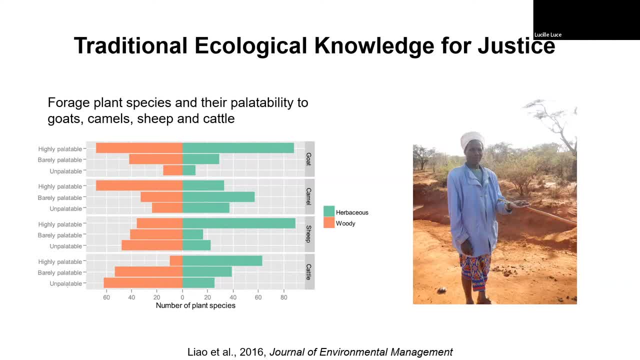 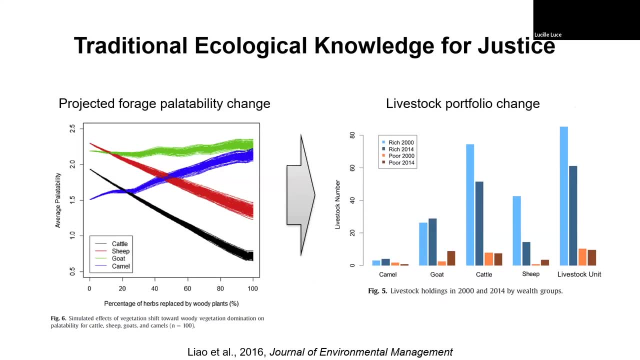 we ask the herders their palatability level to the livestock species And, based on their, based on their like description and also their perception of their either increasing or decreasing in their availability right. We simulate that The plant palatability change over time. 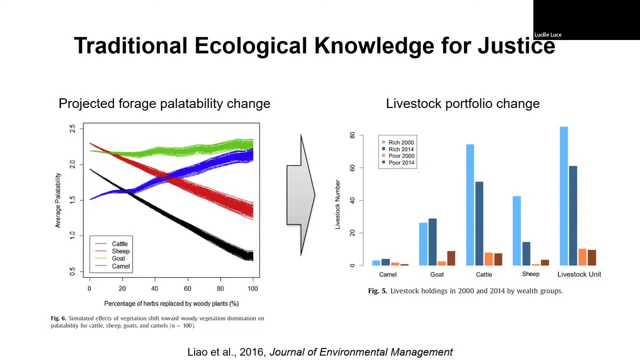 as more herbaceous plants are being replaced by woody plants And we do see that right for cattle is black Cattle and sheep. they will suffer a decline. average palatability Goats will stay more or less the same and the camels. 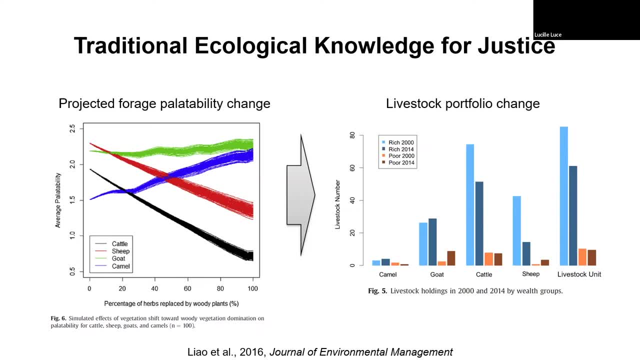 will have a positive change in palatability over time. So actually those, as we can see here, the herders are already adapting their lifestyle portfolio according to their understanding of um, of um, their the plant dynamics change in in on the rangelands and actually i would say this is a, this is um, not a small deal, because um cattle has very important. 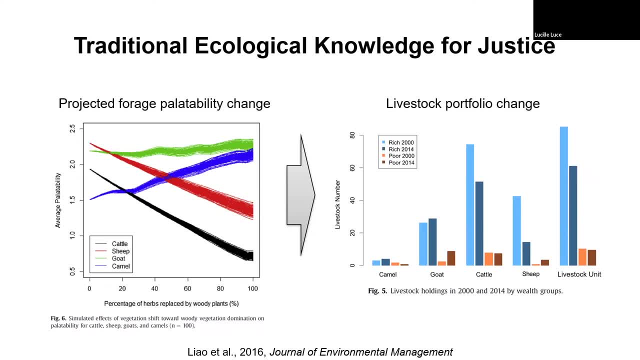 cultural, like significance in that part of the world, the entire, like the, the herding, like the community. the boron culture is built on cattle. now you, if you're asking them to change in in their lifestyle species, it's um, it's a, it's a, it's a big change in their in, not just in their choice of. 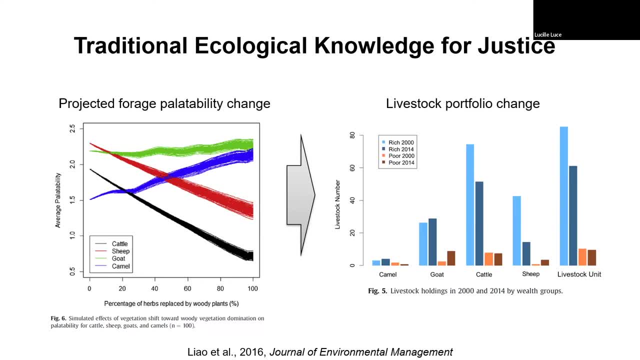 livelihoods and hurting strategy, but also cultural change. but encouragingly right, we do see that um, there is a change in lifestyle portfolio, like especially um, for both rich and poor households. there is a reduction in the amount of cattle that is being sold to the herders and the herders are 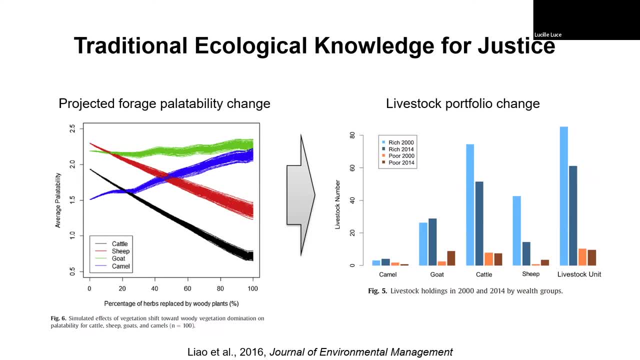 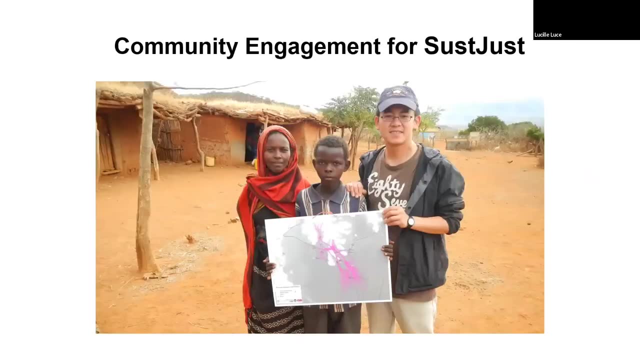 able to increase their cattle with holdings and also for um. but for for goats we see that both groups there is an increase in the holding of gold and for we also households they're they are able to increase their camel holdings and also community engagement right. this is also very important. so i created those um. 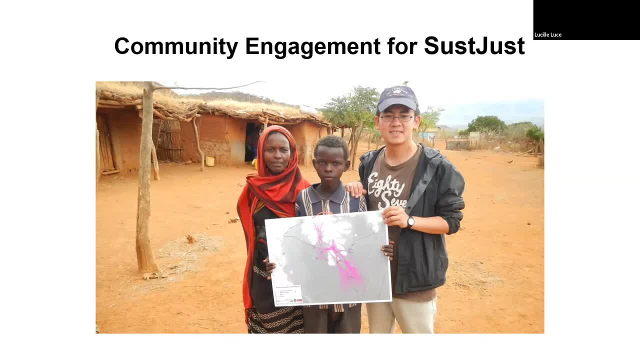 you with this gps tracking data. i created those maps and uh translated them into the local language, often oramal, with my the help of my local collaborators and prindle, and given those back. i gave this maps back to the community, so hopefully those maps will serve as tools to help them. um, help them. 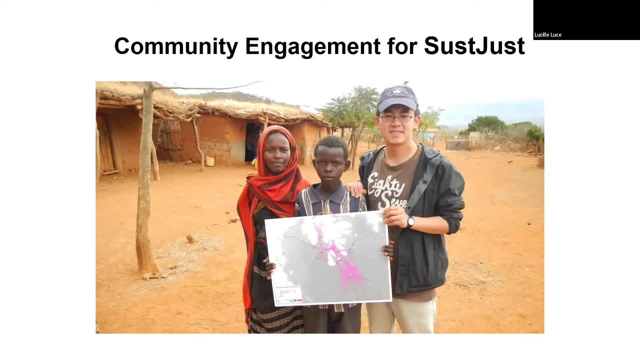 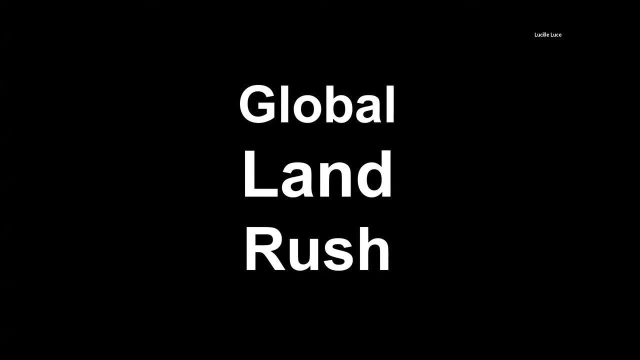 reflect their resource use patterns and and defend their land tenure from potential land grabbing rights, because they're encroaching interest from agribusiness on those lands. so speaking of land grabbing leads to the second topic. i'm not sure. like we have time until 1: 15. okay, i'll go a little faster now. okay, 1: 15 is four questions or just me. 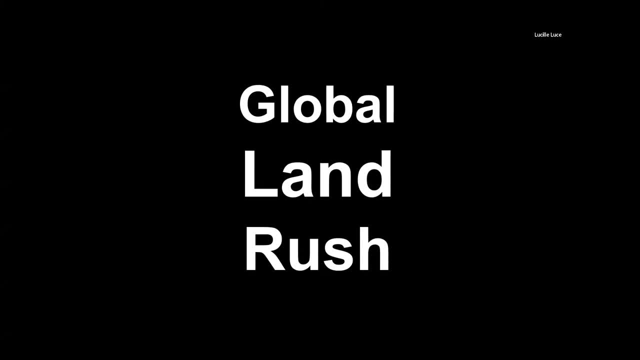 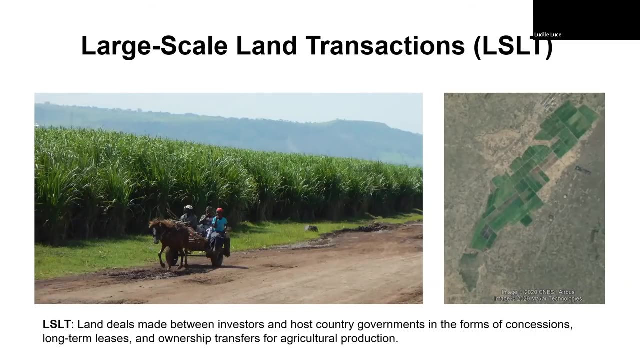 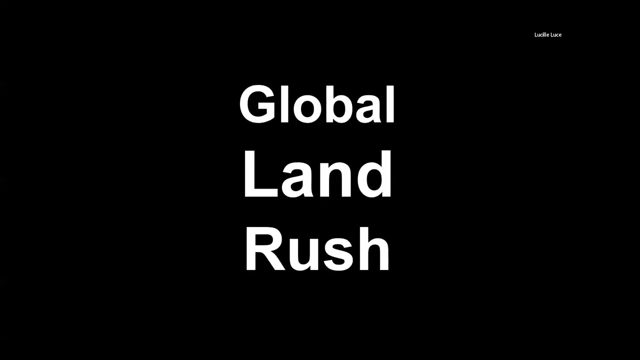 okay, okay, okay. global land rush, the second empirical component, and so what i mean by so here, when we global land rush is a term that's used by like uh me, like media or like um some scholars, but here we are using the term um large-scale land transactions- to refer to the topic, because, like land rush means that it has. 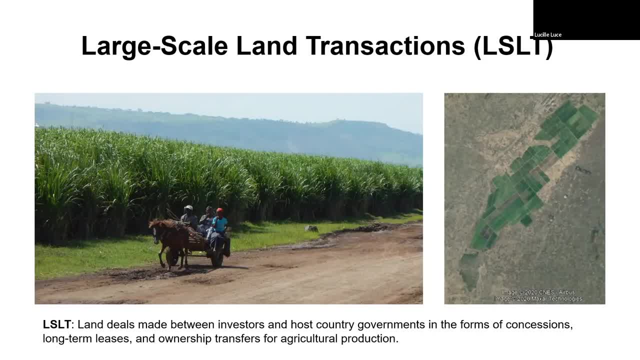 some um, negative connotations and um, even like even worse terms could be like land grabs, right, that that is like focusing on the role of investors, like going to the communities and get land. um, so here we use a term: transactions, because they're not just land grab and then they're also land 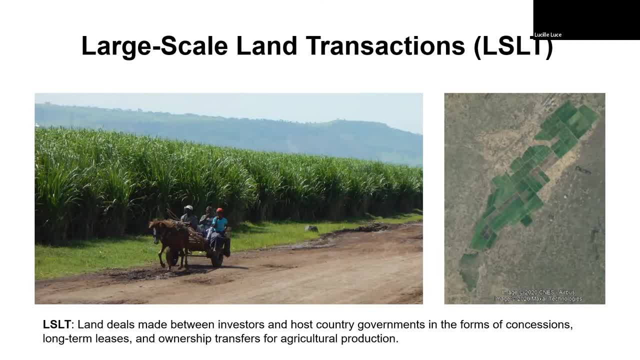 we believe it's more neutral. so this means land deals made between investors and host country governments in the form of concessions, long-term leases and ownership transfers for agriculture production. this is what we are, we focus on here. so this is on the left is the photo that i took. 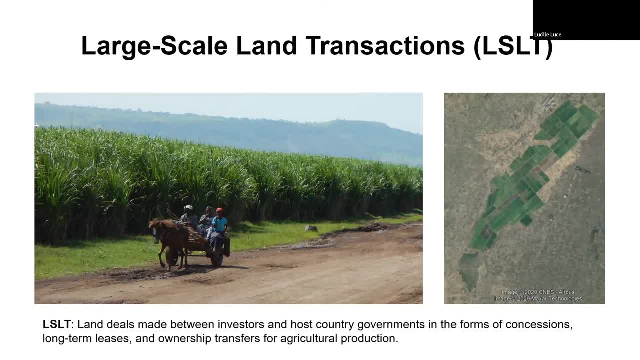 on the ground in uh. so what is this crop? can can anyone easy sugar cane right? it's a large sugar cane plantation, so i was probably somewhere here taking the photo. so you see this large sugar cane plantation starting, like contrast with the neighboring small parcels of a small smallholder. 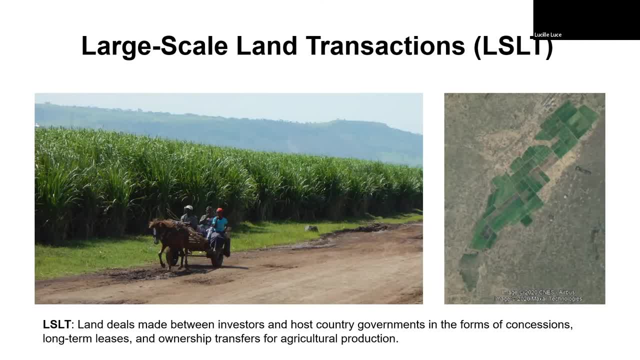 taff or maize patches of smallholder farms. so this is a farm that's built like by aggregating smaller farm lands together and do irrigation and bring water into this area and then and then start the sugar cane plantation. so that's just one form of our land tenure change. 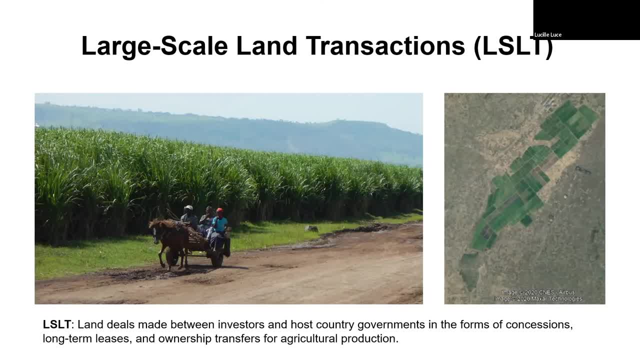 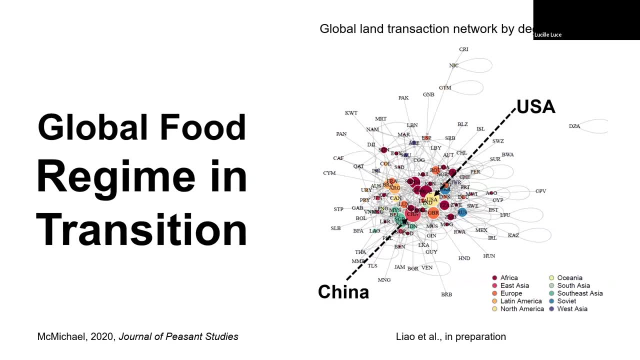 right. there are different forms like changing from like forests, like uh or community forests or like range lands into this kind of large-scale agriculture. so if we look at this phenomenon globally right, the global food regime in actually in transition. we see like um major investor countries go into um to the global south right to to look for land for agriculture development. 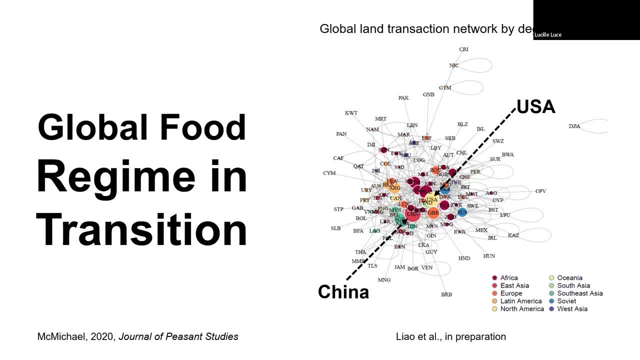 and if we just um use a network approach to understand what's going on, we do see that both us and china, they are the two most important uh land investors in the global land transaction market, right indicated by the size. bigger the size, the more important. that means the higher. 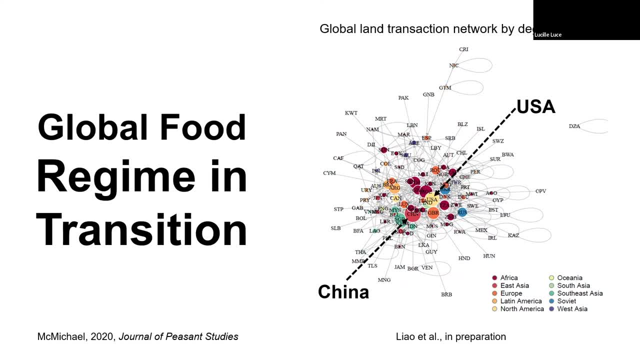 like, the more, the greater amount of land transactions and the the location right in this network means that centrality right they play central roles in this global land rush. so sometimes, like i see star um like in, they blame china for this. our us is doing the same right. so in, at least this is what um the data reveals from this uh. 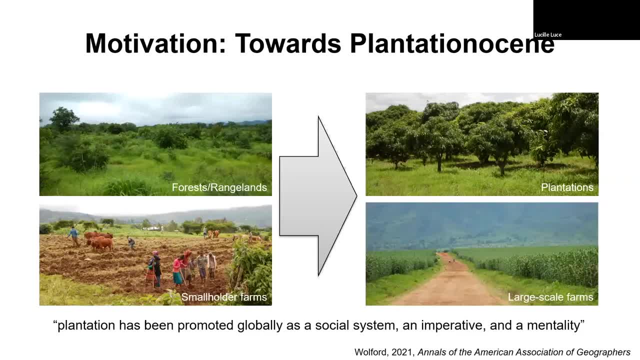 land matrix data set. that's open access. so motivation: why do people want to do that right? so what's plantational things? so this is a paper by my colleague in global development. um so wendy. she argued that plantation has been promoted globally as a social state. 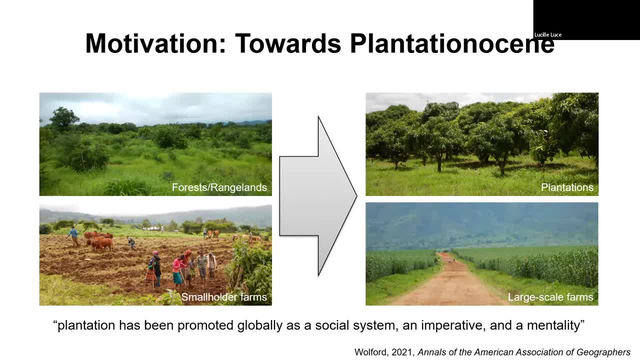 so what's? a paper by my colleague in global development? um so wendy. she argued that plantation has been promoted globally as a social state, an imperative and a mentality right. so in plain words, right. investors want to convert this kind of a they call underutilized forests or range lands into all these smallholder farm plot. 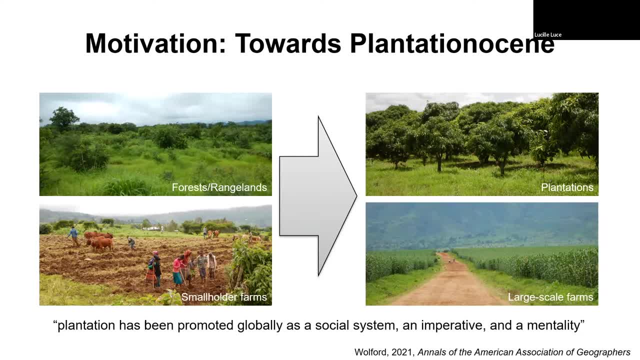 farm plots into this, plantations and large-scale farms right to, and also the local government also has an incentive to facilitate this because this will generate less. this is the mango plantation right intended for for export, so that will generate, like um, foreign currency for their government. 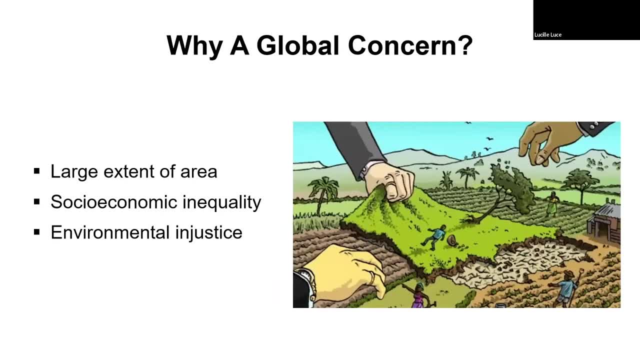 That's very important for them And why this is a global concern. I would say three major reasons. One is large extent areas, somewhere between 40 to 120 million hectares of land. Even the lower end is greater than the size of Germany. 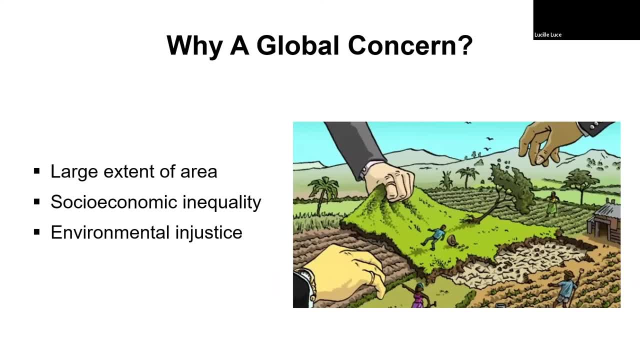 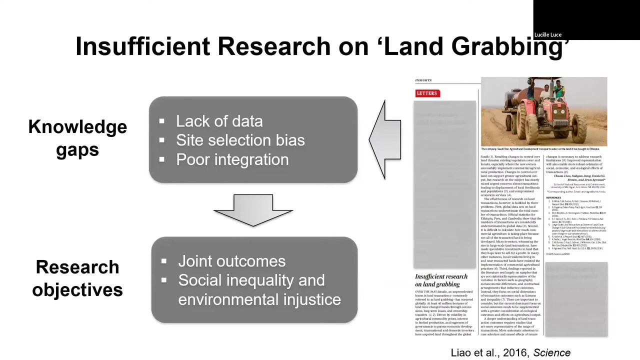 And socioeconomic inequality, as indicated here. right- Agribusiness investors competing with local people for land use And the environmental injustice, like deforestation and the carbon emission associated with this land cover change process. So insufficient, why there's so when our team started to study this issue, right. 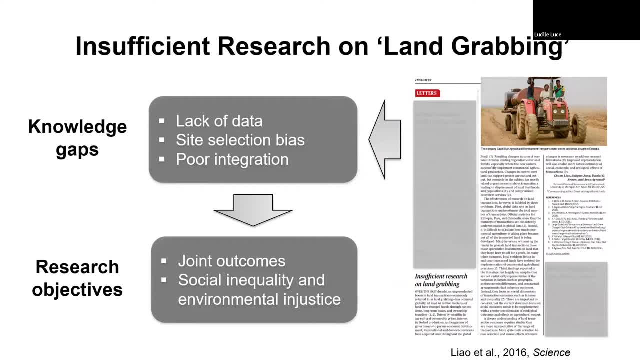 We did a comprehensive literature review and we find the three major knowledge gaps in this topic. One is lack of data, Because land transactions is very secretive- It's government and local investor and the investors make a deal. Usually they don't publicize. 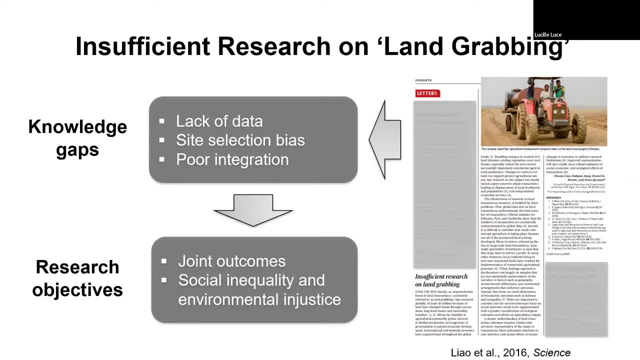 So for scholars it's very hard to access those data in a systematic way And size selection bias- those who are like- cause media headlines. they are more likely to receive scholarly attention And also pre-integration of outcome. So here is what I mean. 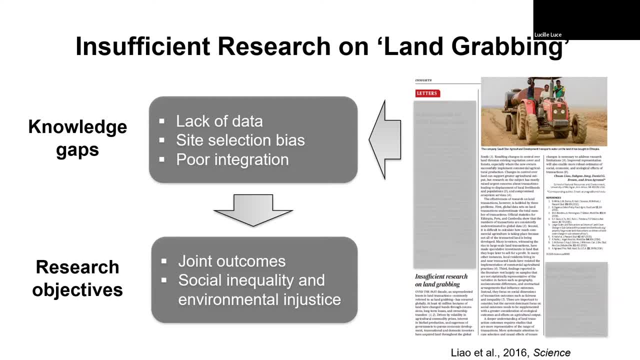 Most academic research, youngest scholars, faculty and on this topic, focus on the social aspects And some on the ecological environment, but there is a lack of integration of socioeconomic and environmental outcomes. So that's why, when we started to study this topic, 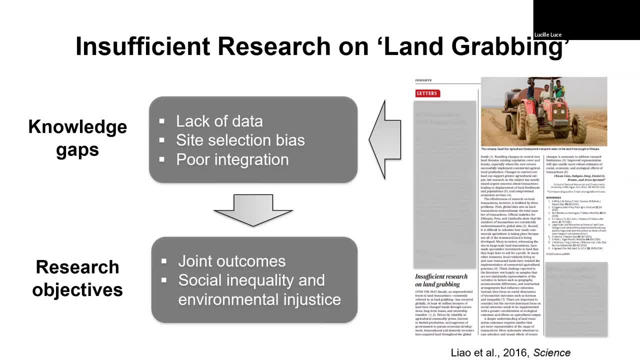 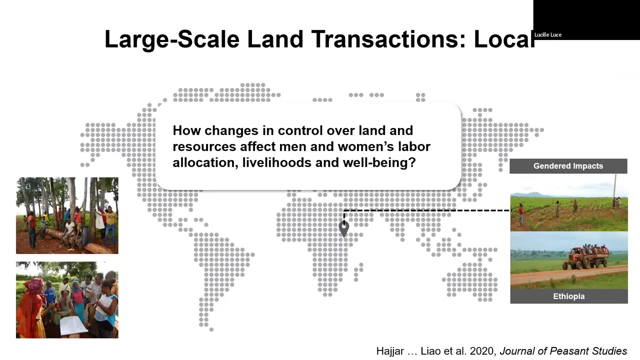 we decided to focus on the joint outcomes when we analyze this, and with attention to the social inequality and environmental injustice issue associated with land tenure change. So I studied this at different scales, at the local level. So we answered the question of how changes in control. 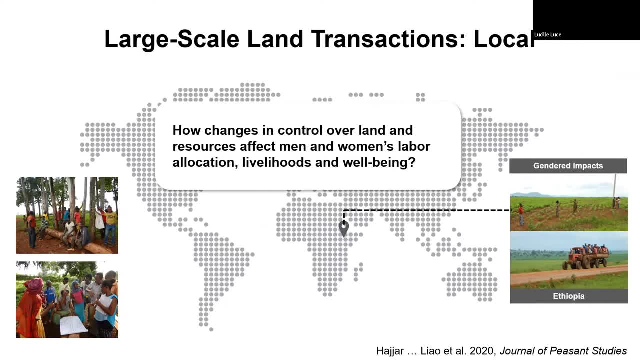 over land and resources affect the men and women's labor allocation, livelihoods and well-being. So when we were in the communities we do see men and women were treated differently. Both of them work on the farms, but women have to take a plow, carry the plow by themselves. 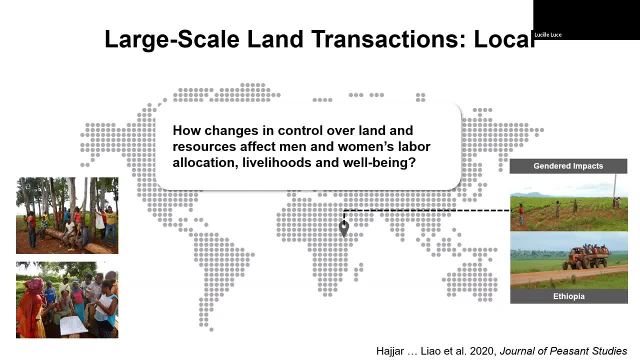 and walk to their assigned farm plots to work, But men, at least they will have a tractor to transport them from the village to the farm plots. That's what we observed at first, And then we held a different focus group discussions with male and female groups to understand this. 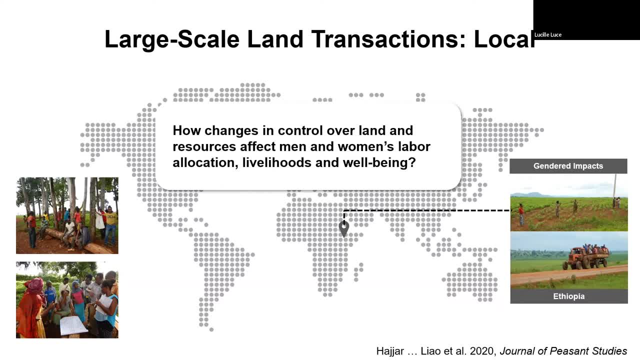 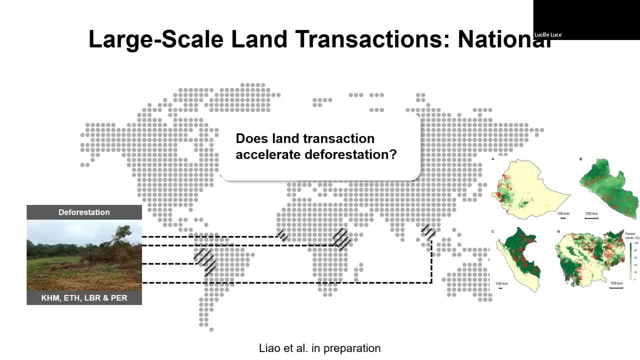 So here I'm not going to talk about the details, but just to give a sense of at different scales we answer different questions And the national level. so we answered the question of: does land transaction accelerate deforestation? So we answered the question of does land transaction accelerate deforestation? 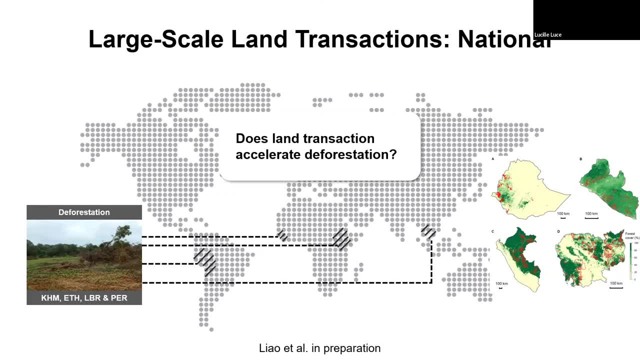 So we answered the question of: does land transaction accelerate deforestation? The important thing is accelerate, Because even if a land transaction doesn't happen in those areas, the growing rural population in the developing world may also cut down forests to grow more food right. 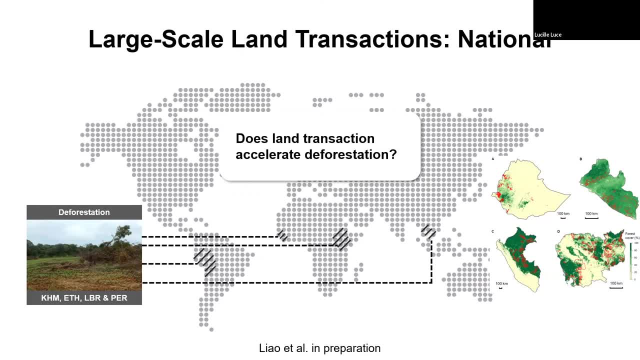 So the point is using an econometric approach to do call the inference on whether land transactions accelerate deforestation. So here we focus on deforestation. We focus on four countries- Ethiopia, Liberia, Peru and Cambodia- where we can get land transaction boundary data. 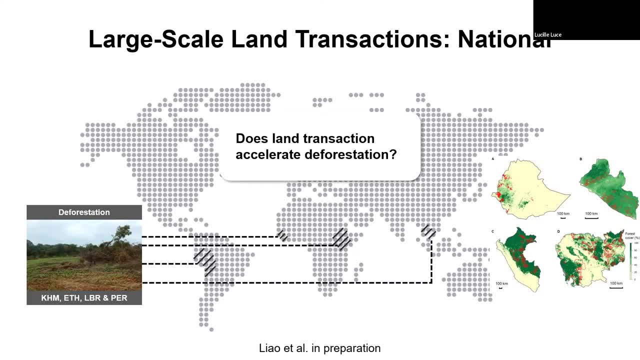 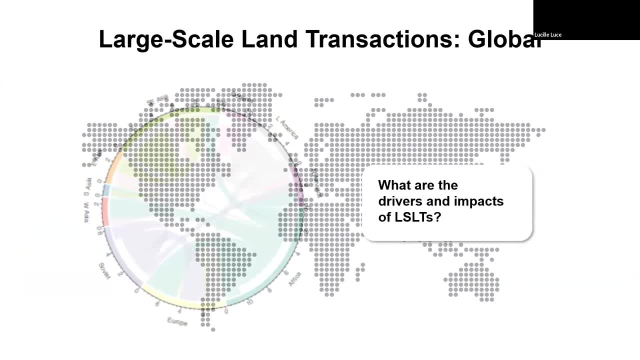 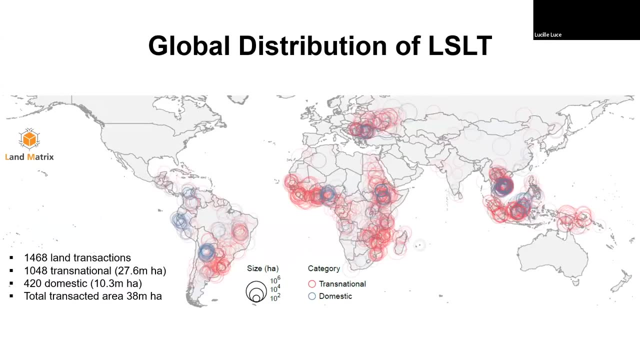 the polygons right. So, as I said, this is very hard to get this kind of data because of secrecy of those deals And the global level. we studied the drivers and impacts of land transactions. So for this one I'm going into a little bit more details. 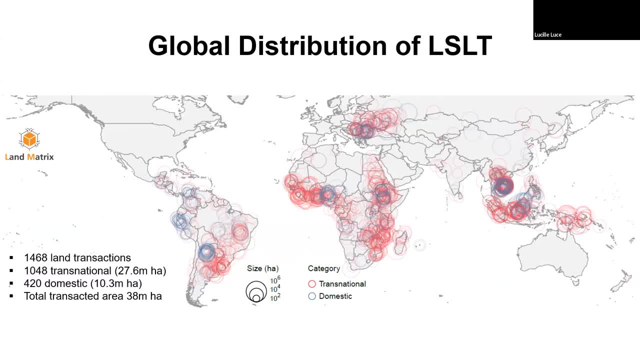 So first, global. so this is a data source that I mentioned to generate the network right that I mentioned earlier. It's from this open source data set called the land matrix. At that time when I did the research, that's about 2016,, 17, right, there are about. 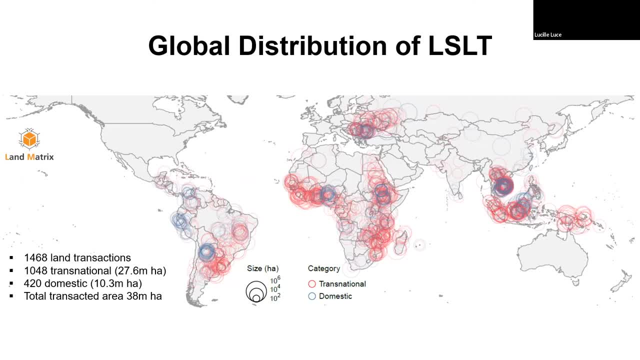 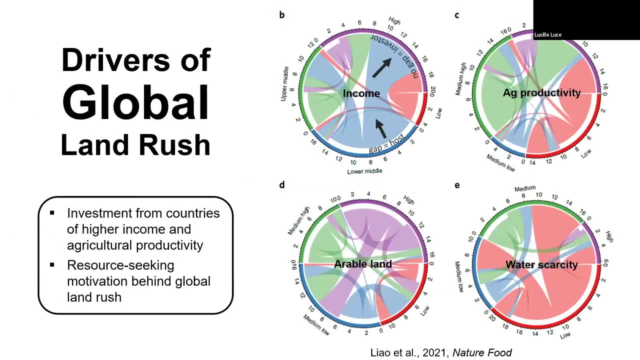 1500 land transactions globally, like as you can see the distribution here. So with this data set, we first analyze the drivers of this global land rush by comparing the characteristics of investor and host countries of land transactions, right according to like per capita. 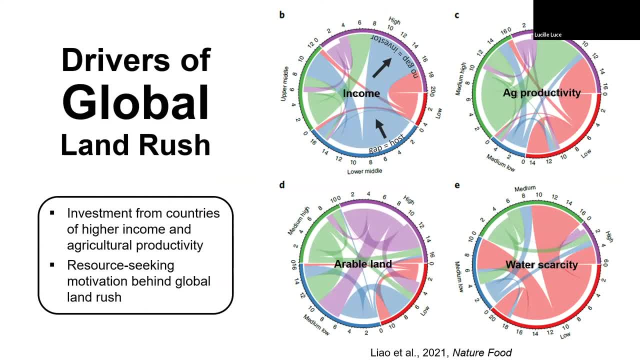 income, agricultural productivity, arable land availability and the water scarcity. right Across those four dimensions, we do see there is a flow of, like a virtual flow of land right from wealthier, from less wealthy countries to more developed countries. 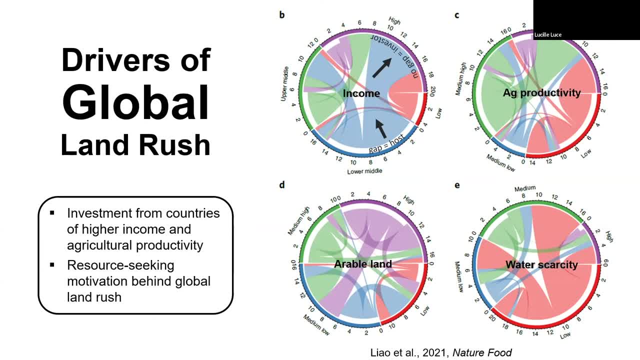 right, as you see, low-income countries. they indeed predominantly serve As a supplier of land in the global land rush. So because of time, I'm not going to all the details in the other three, But what is a more important question is right. 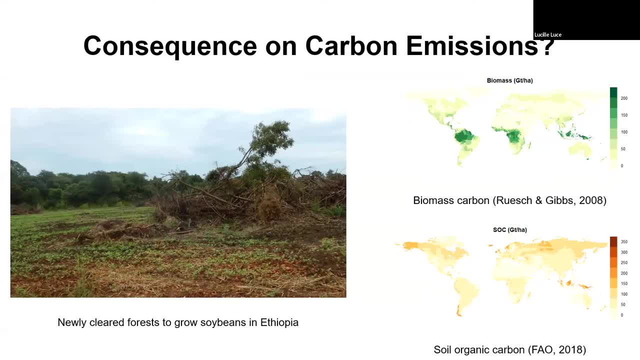 the consequence of this, Like there are many studies on deforestation, but so that's why I think, but carbon emissions from this process hadn't been studied that much. So that's we see that our potential contribution, and we only studied the issue at emissions. 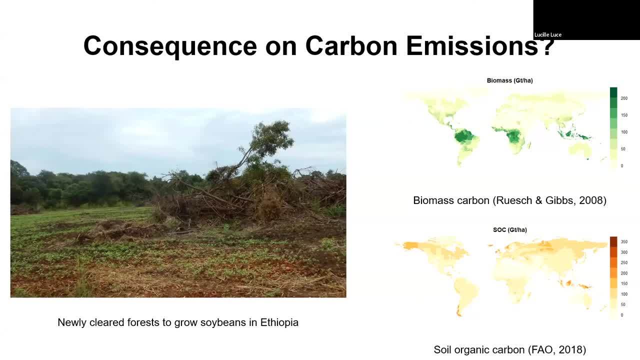 at the land conversion stage right, So it's a long supply chain And then it can have have like more carbon generated from this process here. This is just a represents a starting point, which is like a quantidade use conversion. This is what I took in Western Ethiopia. the photo: 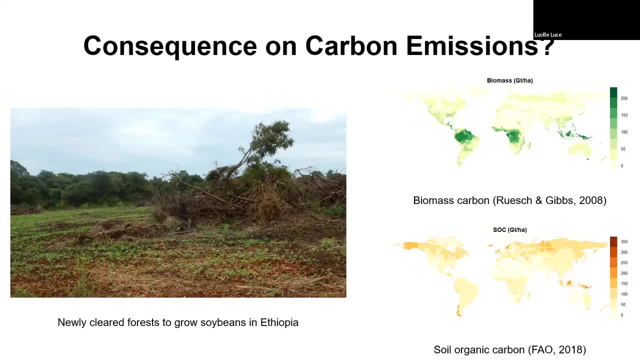 So it shows like this newly cleared forest to grow soybeans in Ethiopia. You see the cleared like woodlands, it's yet to be like burned. And then you see those soybean seedlings on those lands And there are two major sources of emissions right. 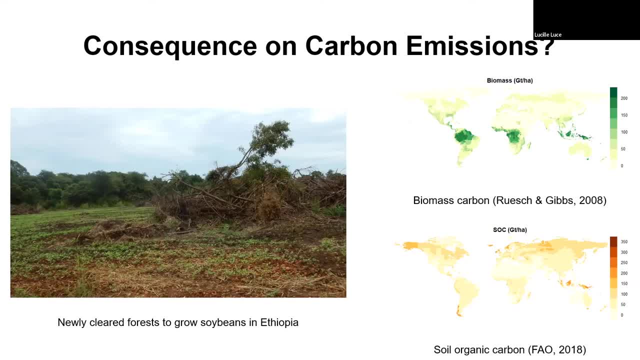 At this stage, biomass and the soil organic carbon. So there are some globally available data sets that we use for this estimation. Although biomass carbon right, once you clear they are all lost. but soil organic carbon loss is a different story. 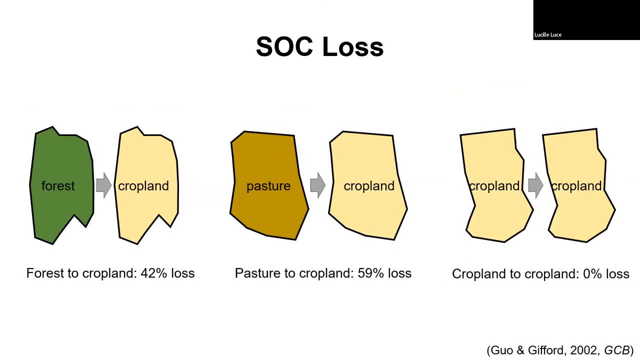 So we refer to the literature. I mean, this is just the average number, right, Because at different locations the percentage of loss is different. right From forest to cropland: 42% loss. Pasture to crop: 95.. 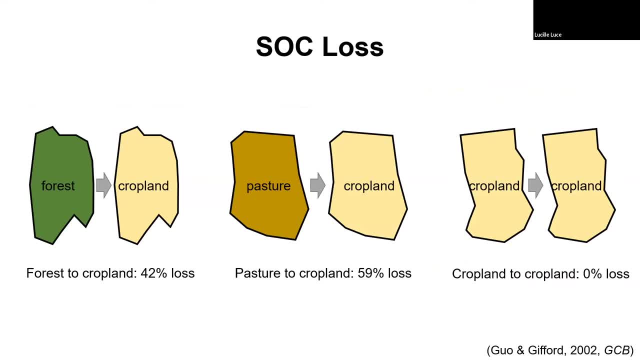 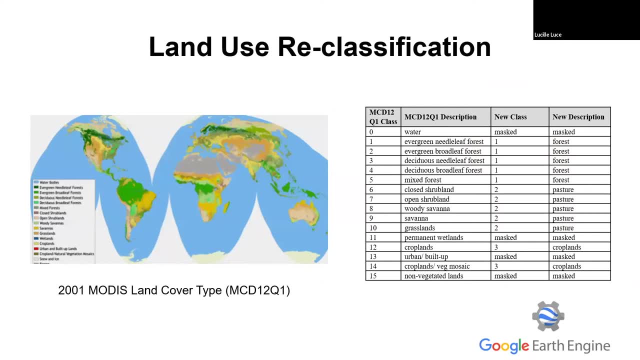 And crop to crop, like smallholder crop to large-scale crop, right, 0% loss. So with that kind of variation taken into consideration, then we need to think about, when we change, what's the starting point- land cover- and what's the ending point- land cover. 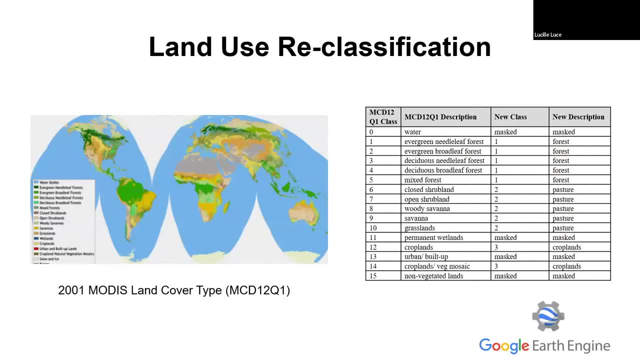 Ending point it's clear it's cropland right, But starting point we need to. so here we use the 2001 MODIS land cover global data set to do this land use classification using Google Earth Engine and master water. 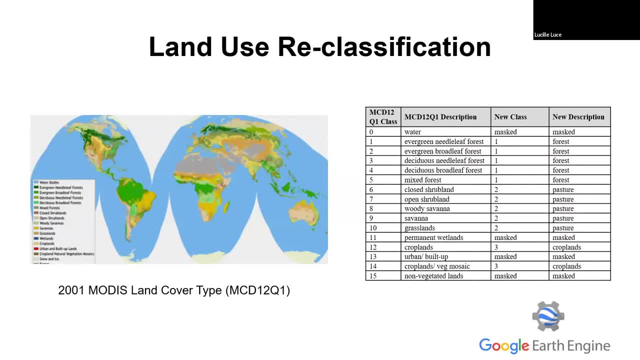 permanent wetlands, urban and non-vegetated lands, because land transactions are unlikely to happen right in those areas, So we need to exclude them. Probably, in retrospect we can exclude more areas like such as by considering the slope. 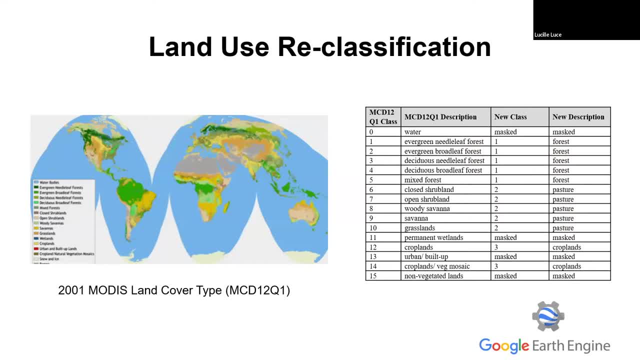 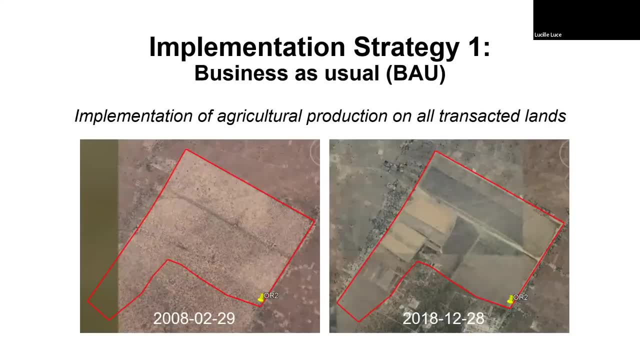 or some other environmental covariates. But this is, as I said, it's just representing like our first step to answer this question. So then we need to consider about the implementation strategy, right? The first is the business as usual, right? 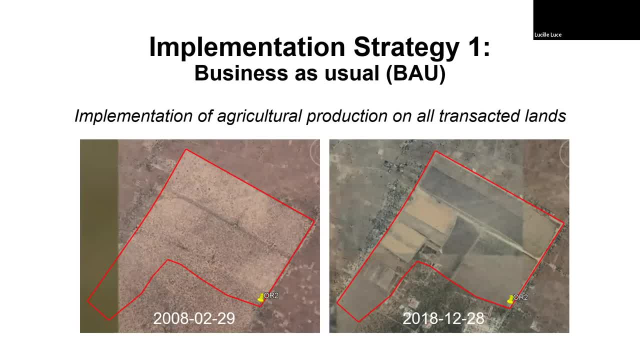 As an investor. you would clear, all right, you would clear all the lands to maximize your economic return. right Convert this. this is in central Ethiopia. This is a sort of a typical savanna landscape. You see there's some tiny tree canopies. 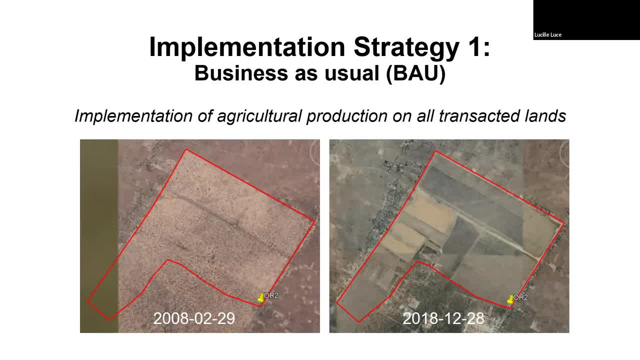 sparse tree canopies have been come, but then after implementation they are all cleared. to establish these large-scale farms right As an investor. you would do this. And then this means for forest pasture and whatever landscape the prior landscape is. you would do this. 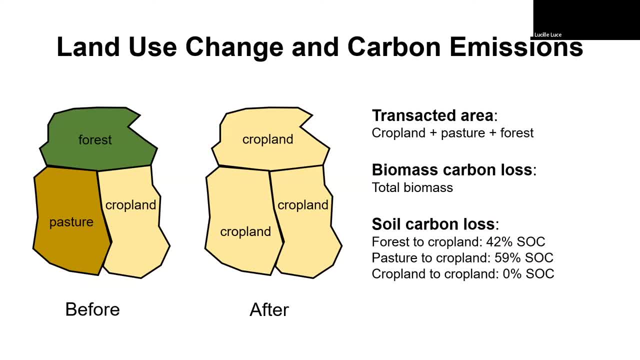 And then this means for forest, pasture and whatever landscape the prior landscape is, you convert all of them into cropland And then, based on this scenario, we calculated the total transaction area: biomass carbon loss and the soil- organic soil carbon loss. 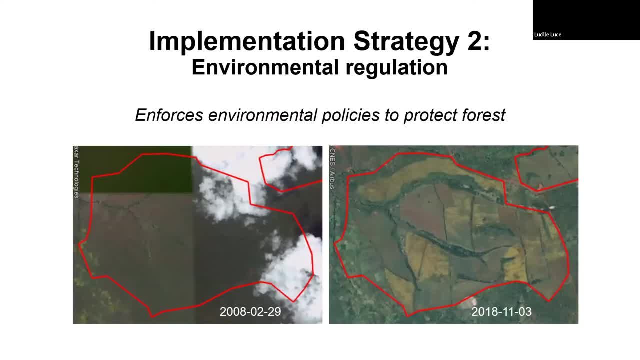 But what's the next strategy is what we propose, as that can be used as a policy tool to reduce carbon emission from this process, basically to enforce environmental regulations to protect forest. But then this is like, then the question, the challenge here is what kind of environmental regulations? 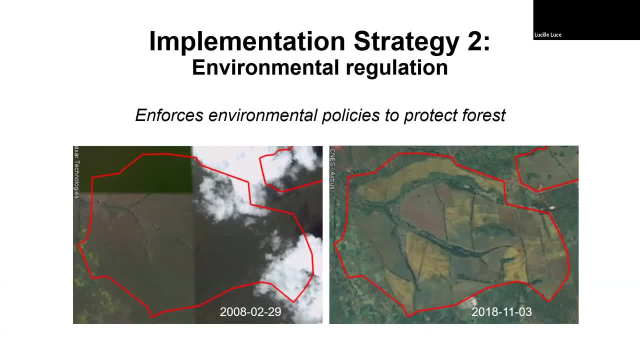 and how such regulations can be enforced on the grounds throughout the global tropics. That's our challenge, right Even if, in Ethiopia, let's say, the central government say you need to retain at least 20% of natural vegetation on the landscape. 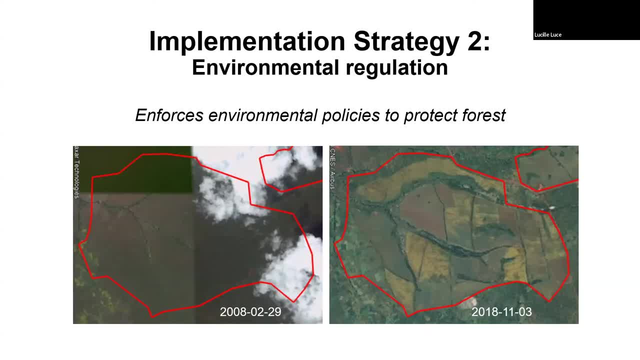 But when it comes to ground implementation, it can be very different. It can be very different across different regions. So that's why what we did is like to apply the first administrative unit level- deforestation rates in the past 15 years- as the level that can be enforced. 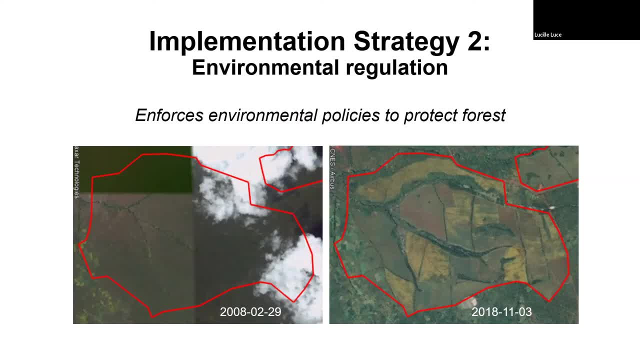 on the ground to determine the level of the enforcement that we can do like globally right. As you can see here on the right side, we do see some natural vegetation that is being retained. on this land transaction side At least, this is a good example. 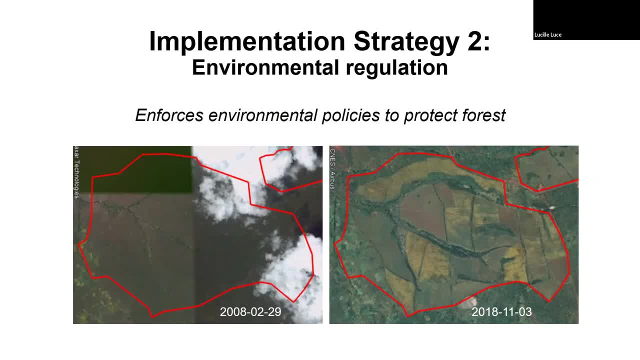 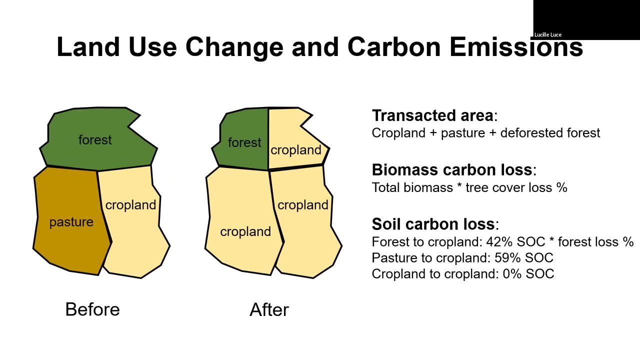 This is better than cutting all the natural vegetation, right? So then this diagram shows the before and after. So that means, like for the forest, we retain whatever level that can be enforced on the ground and see how much carbon emission that we can reduce. 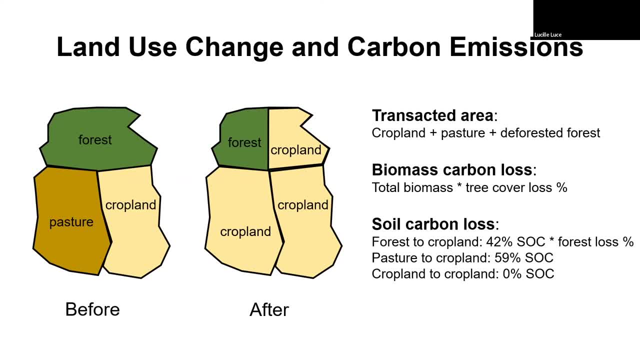 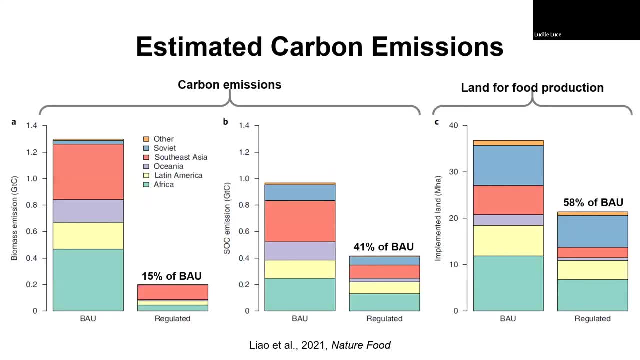 Then again we use a Google Earth engine to determine the tree cover loss percentage and the forest cover percentage. So for the technical parts- I'm not going into the details And just a little bit more here. this shows the main results, right. 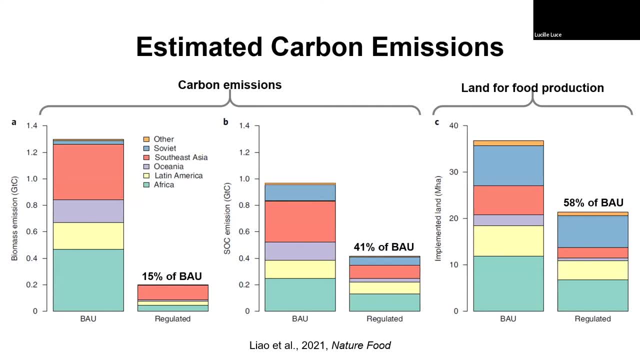 It's about synergy. In this case it's not necessarily about the synergy, but it's more about managing the trade-offs between emissions and agricultural production, As we can see here. so if we change from business as usual to regulated scenario with some like meaning, enforcing environment, 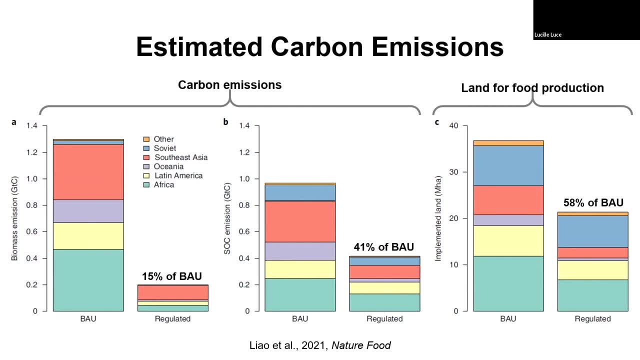 of forest protection policy, Then biomass emission can be reduced to about 15% of the BAU scenario and soil organic carbon loss can be reduced to about 40%, But at the same time nearly 60% of transacted land can still be implemented for agricultural production right. 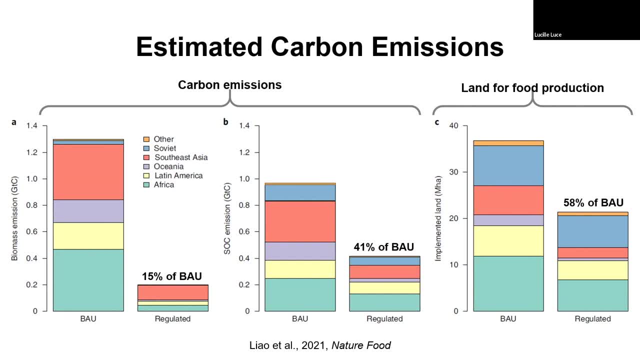 So this means, like if we need to recognize both goals: carbon emission And also food security, especially in Africa with growing population, we do need to produce more food. The question here is: where do we decide that we can let this kind of capital driven agricultural? 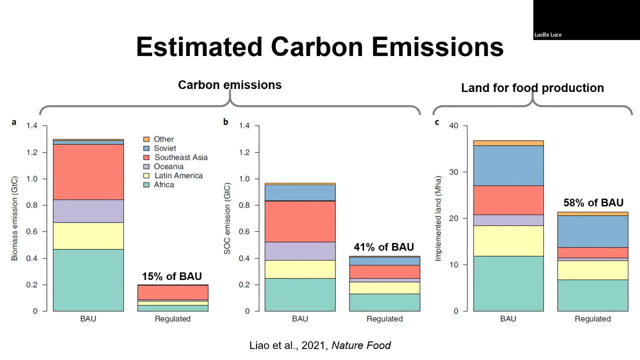 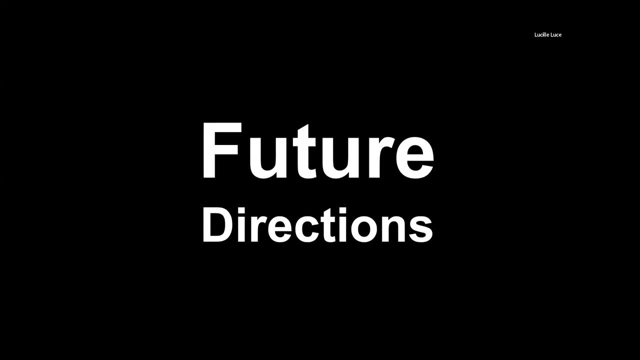 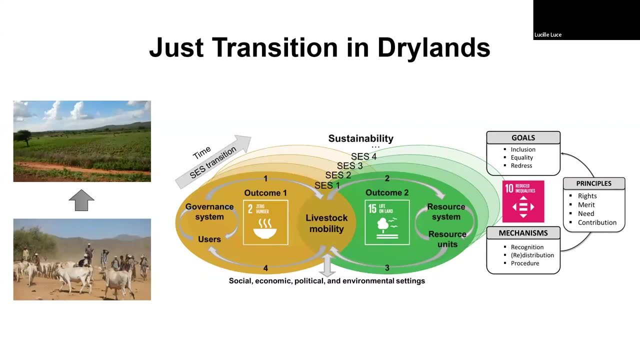 development to happen And, at the same time, we save those high carbon value forests? right? That's the main message. So I will just spend the last two minutes to briefly talk about the future. Future directions: right, One is built on my first topic that I talked about. 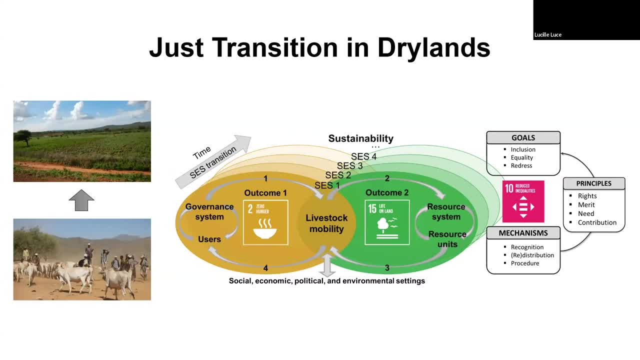 is the just transitions in the dry lands right As the system transition from this into more like crop or like more like a cropping system, from this herding to cropping, then How can those herders, like the local people, adapt to those changes? 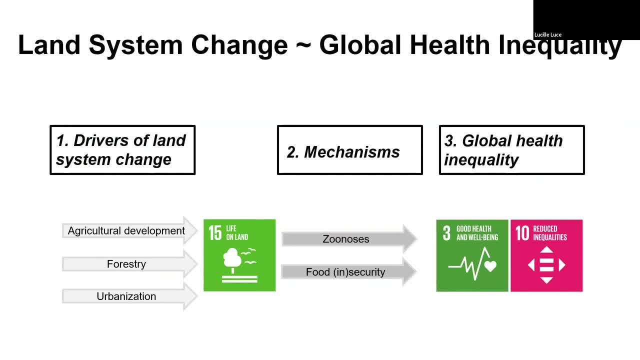 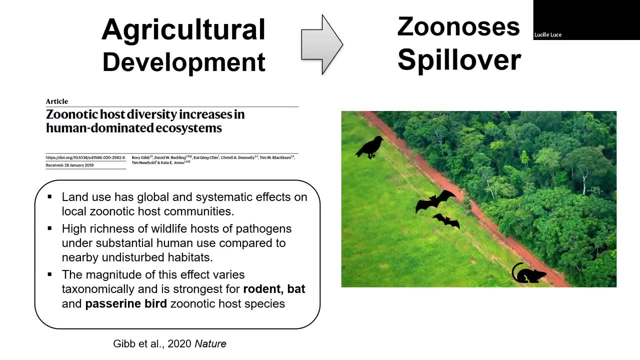 And the second is about land system change and global health inequality. Basically focus on to study the drivers of land system change and two major mechanisms: zoonosis, which are zoonosis spillover, and the food insecurity, and global health inequality, And actually I started to explore a little bit of those. 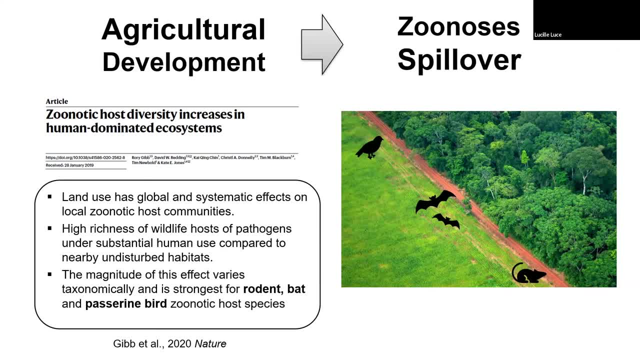 to understand agricultural development and its consequence on zoonosis spillover. right, Because existing research has already shown that major zoonotic disease host issues such as pasturing birds, bats and rodents. They're more likely to thrive at this interface. 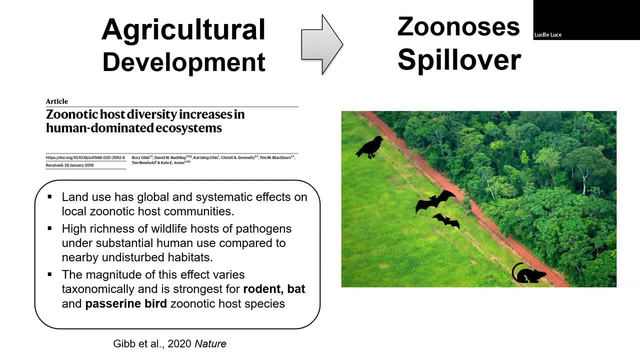 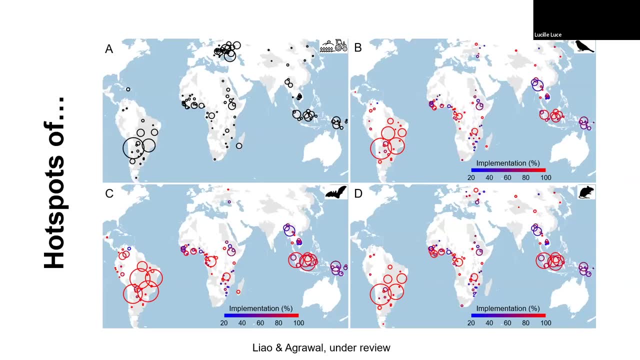 between natural and human-dominated systems. So that's why land transactions are the driver of this. We'll certainly increase this boundary between those. So, at the first step, we are mapping these global hotspots of zoonosis spillovers because of land transactions. 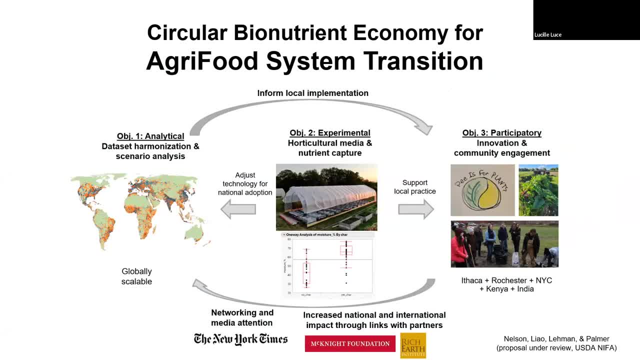 Newtons, Newtons, Two topics that I just started to explore in my first two months back. here is: one is a circular bioneutrinic economy for agro, for system transition One: we have a proposal right now, reviewed by USDA, NEFA. 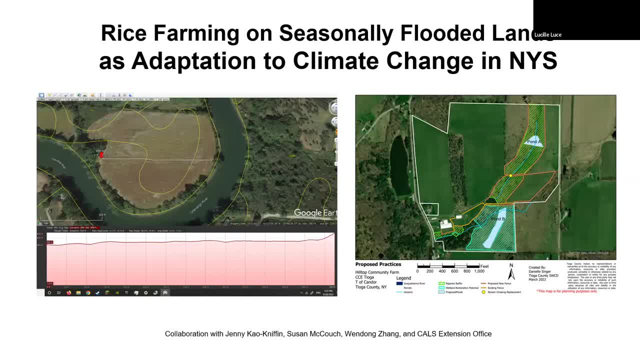 And another potential project is rice farm or as farming on seasonally flooded lands as adaptation to climate change. in New York State, right So, as because of climate change, more in here, they have been seasonally flooded. If we can do rice farming on those lands, 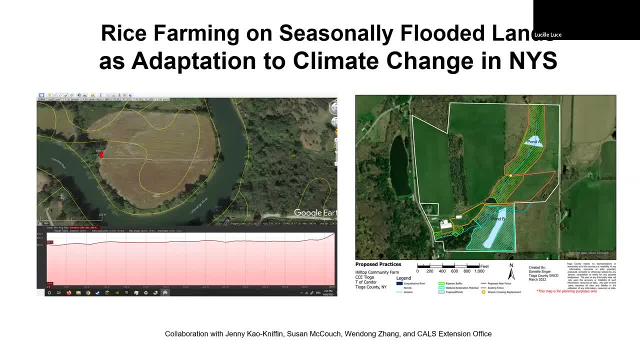 it will turn those kind of- how to say those disasters into production opportunities. So, yeah, again, this is an example of global developments. It's not just about what's going on in Africa, but also here in New York state. So that's it for my talk today. thank you. 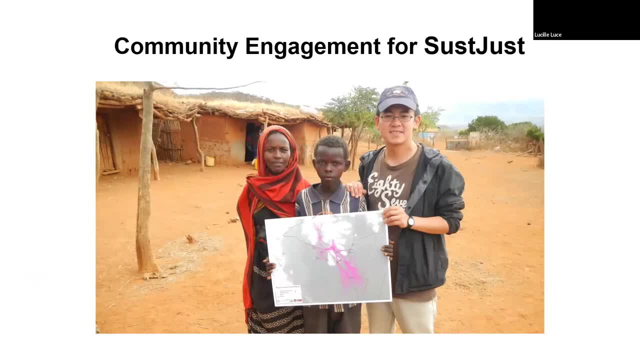 Yeah, Yeah, unfortunately not yet. That was my last trip to those communities. I really hope like we can raise some funds and go back to the communities and see whether those information have an impact, have any effect on their resource use patterns, right, 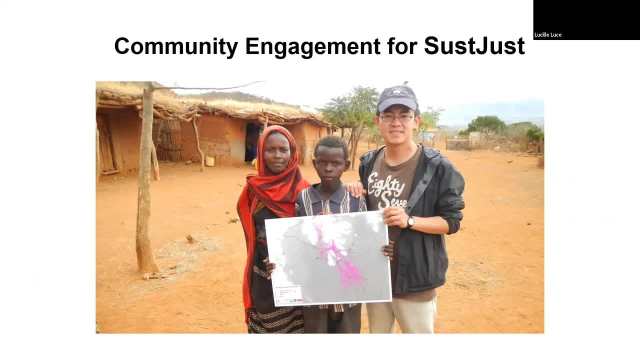 That's my hope, but I really wanna see whether that's having any effect in those communities. Actually, they say the cost of making this map is more expensive than a goat- My local collaborators. they will say: why don't you give them a goat? 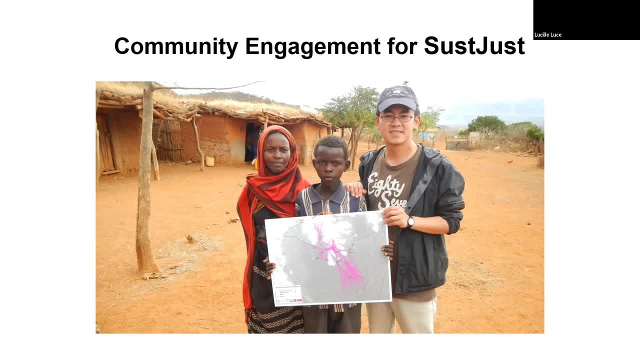 They will be happier than receiving this kind of a piece of map. I said: this is what I can do. But you know the mentality is very different. but that's what I hope. But when I give this map back to the communities, 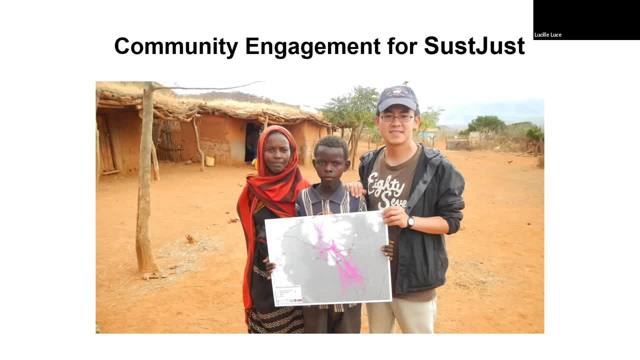 we discuss. right, some of the younger people they can, they can raise, They can read those maps and see: oh, this is a whale that I go to in the dry season. That's our community school. You know they are very good at like a spatial orientation. 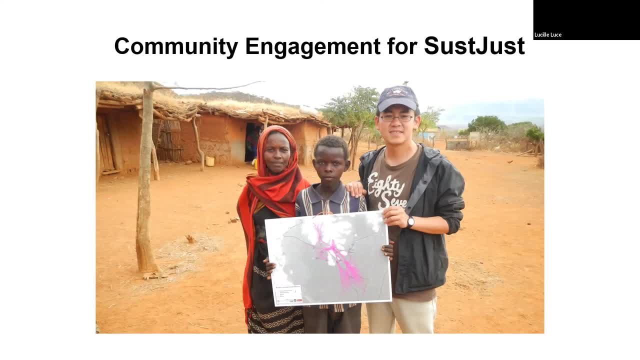 those pastoralist communities. So I do hope that this can have some effect. Yeah, that's a good suggestion that maybe we can raise funds, like seed funds from somewhere to revisit those communities. I'm not sure actually, you can ask Ying. 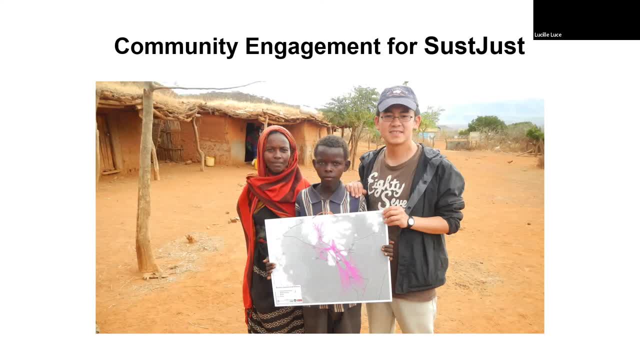 She is working with Chris. I'm curious, those projects- and this is one actually it's one of Chris's, his PI on this- I need to ask him this question actually, if there's any continuation of in this line of thinking. 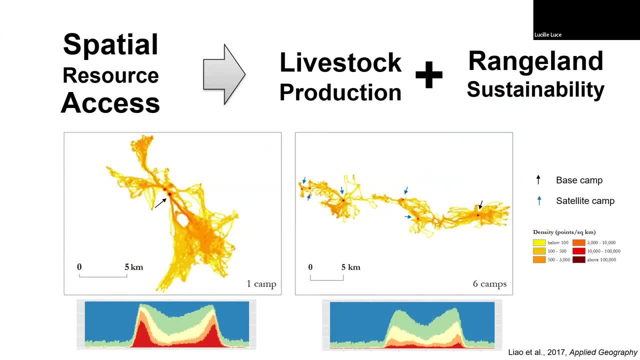 Yeah, thank you. Yeah, exactly. Actually I didn't show some of the maps that are of land sharing. It's like community from like these are at least 50 kilometers away from each other. Sometimes they are like we see evidence of one community going to the other. 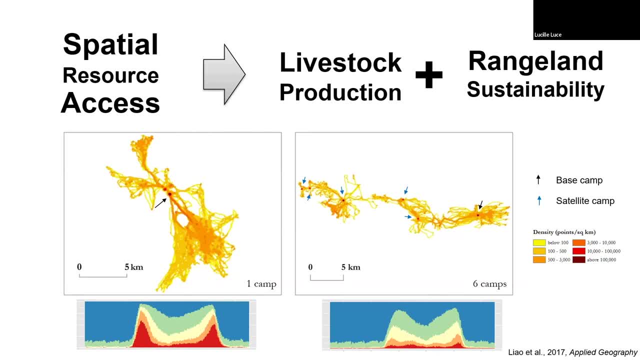 to share land with others. So they are already doing this kind of land sharing on a reciprocal basis. Yeah, the external standing is shrinking for all communities, but these kinds of institutions to facilitate that kind of land sharing, yeah, it's very crucial for them to maintain. 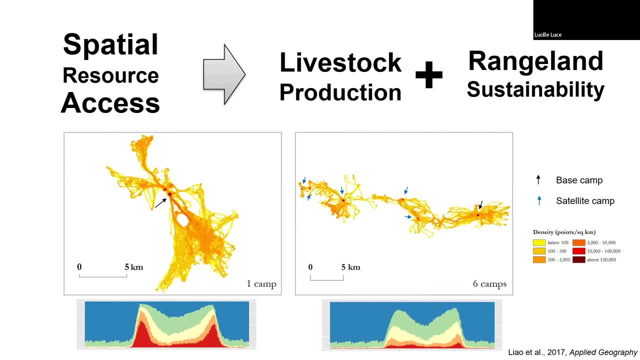 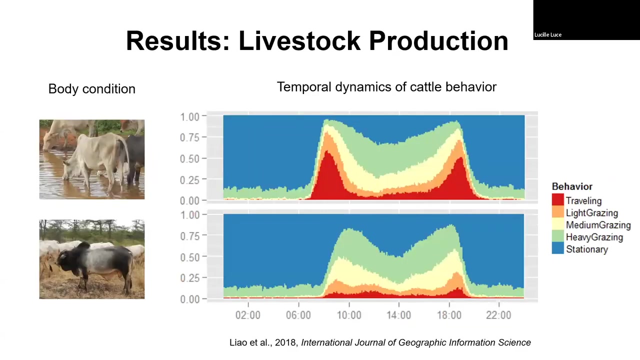 a relatively higher level of mobility? I'm not sure That's your question, or Yeah, I do think so. right, Because at least they can minimize the walking right, That reduce like a stress for the cows right In their daily grazing like activities right. 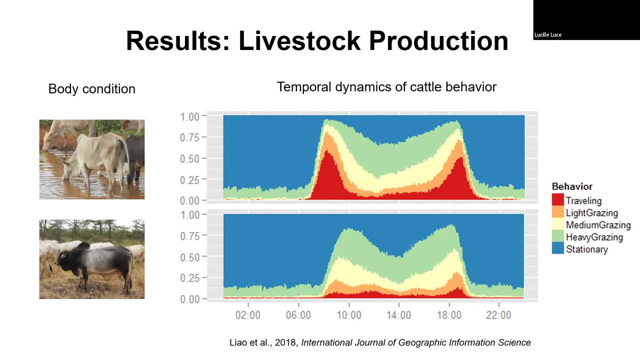 Exactly so. yeah, thanks. So will I, or you, Or is that even more of a debate? Sure, yeah, there is a big literature like on those topics. So from the investor's perspective and also from more from this local people's perspective, 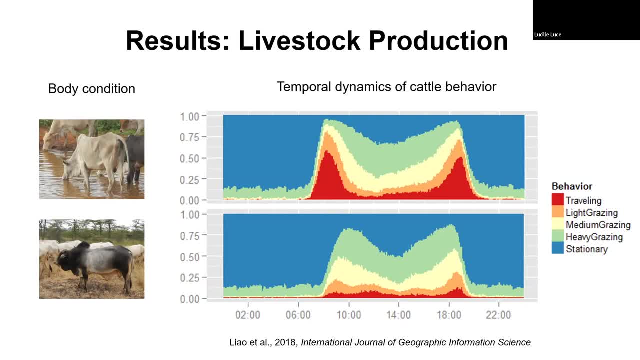 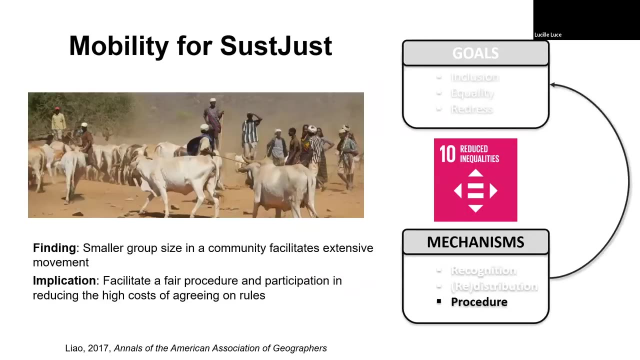 based on my interaction with the local people, they are more than happy to get more involved because that means higher return for them. But once you establish this large scale farm, that means less demand for labor, higher mechanization. Those people basically- let me just use this- 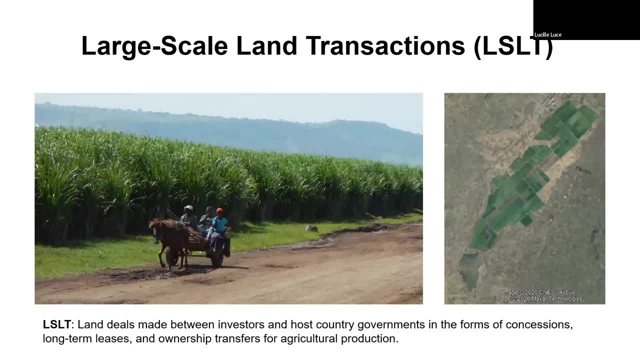 example, for this one, what they received is a share according to Share of revenue, according to their land contribution to this sugarcane plantation. Then that basically freed up the labor within the household that they can go to the nearby towns and cities to serve as wage laborers. 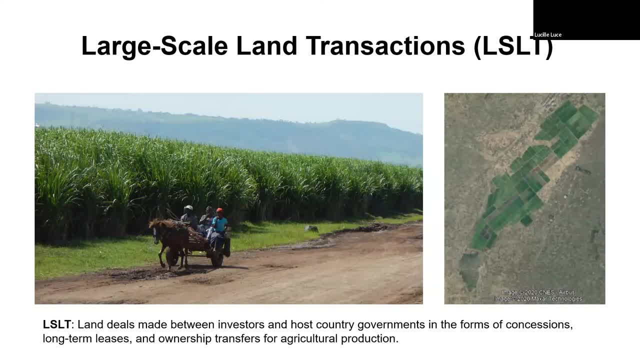 and also all work in the Chinese factory, like there is a Chinese economic just nearby. they just go to make shoes in the company and they earn a wage. So actually, So actually, Local people are more than happy to do that. 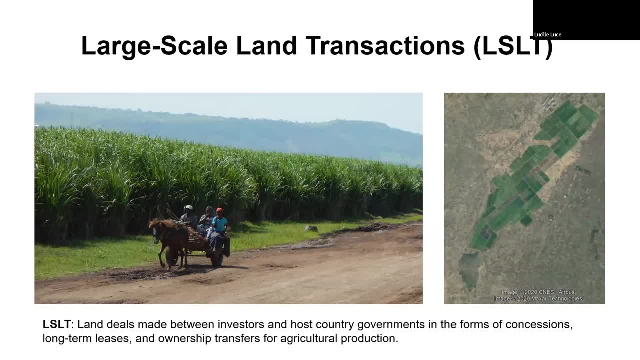 I wouldn't say all of them, but some of them. they are happy to do that, But the thing is lack of opportunities, like the Chinese economic zone, If there are more of those that can provide employment opportunity, especially for the young people in Africa. 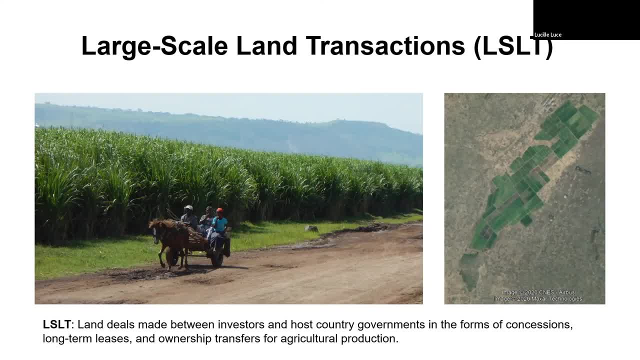 I think this will work out even better. But actually one of the major concerns is, once you do this, what happens to the local people? They lose land, they lose means of livelihoods. They at best get a share of the revenue from the sugarcane plantation. 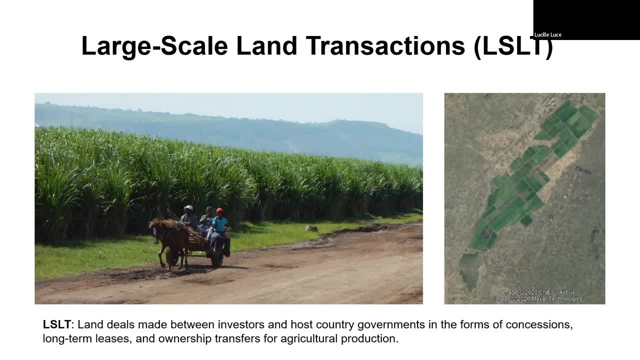 That's the best they can expect Because they don't want to hire local people. And this is in central Ethiopia in the agriculture. But if you go to the pastoral regions or in the sort of the periphery of Ethiopia, then those local people have very little skills of farming.